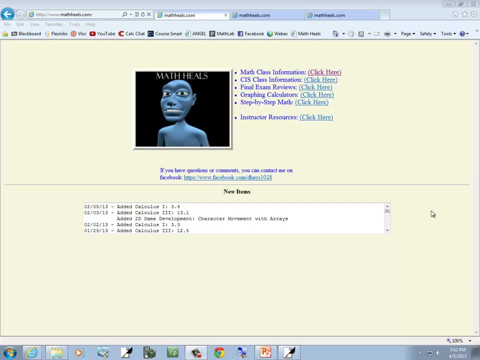 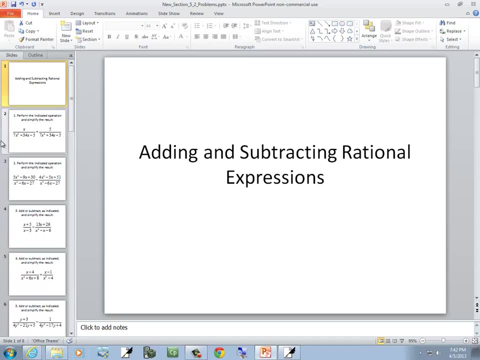 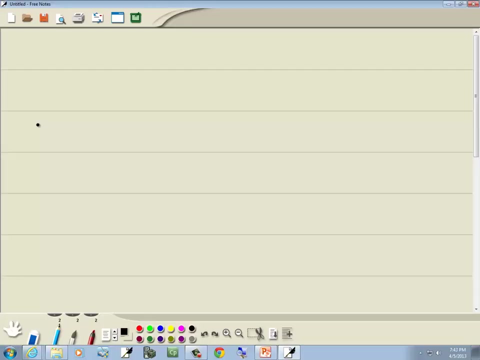 This is mathhealscom, where you can find more links to math and computer science- YouTube videos. Let's take a look at adding and subtracting rational expressions And take a look at our first problem. We got x over seven x squared plus thirty four x. 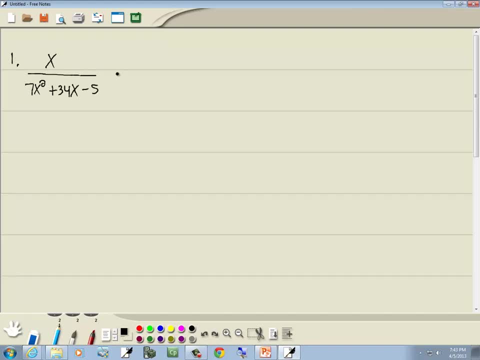 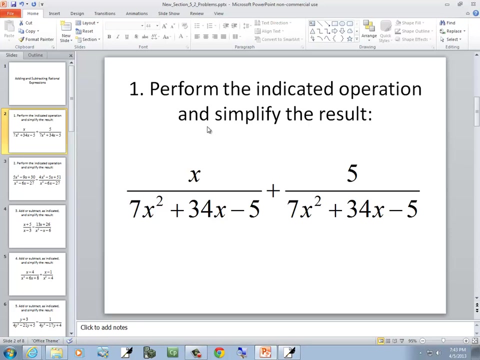 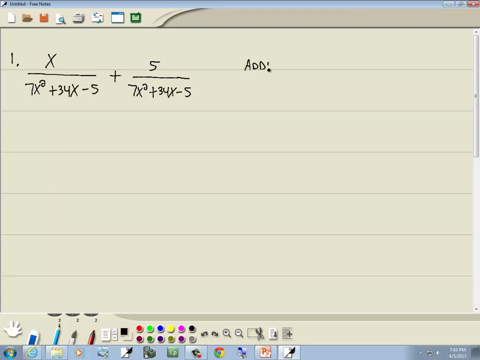 minus five plus five over seven, x squared plus thirty four x minus five. And instructions say: perform the indicated operations and simplify the result. This is going to be adding, subtracting rational expressions with the same denominator. So adding and subtracting rational expressions when they have the same denominator. 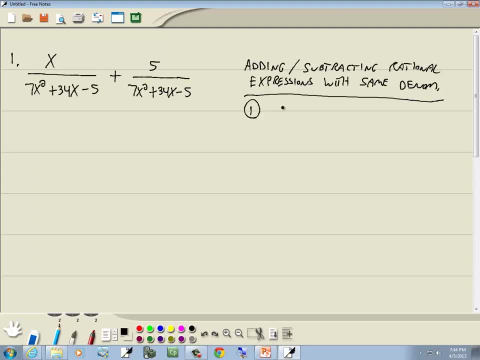 Well, our first step is: we'll add or subtract the top parts, the numerators, and put into a single fraction. So add or subtract top parts and put into a single fraction. Well, here we have a plus between it. so add top parts x plus 5, and then our denominator. 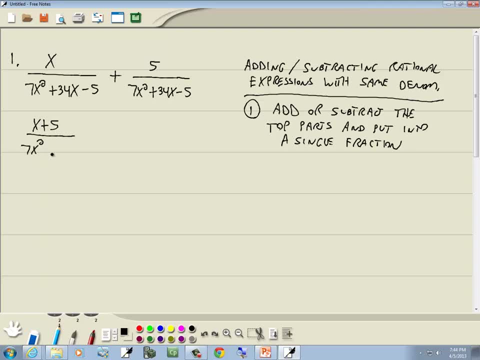 stays the same because the denominators both of these are exactly the same. There we go, Step two: factor the top and factor the bottom, So factor the numerator and denominator. Well, on this particular one, here the top part doesn't factor, but the bottom part does. 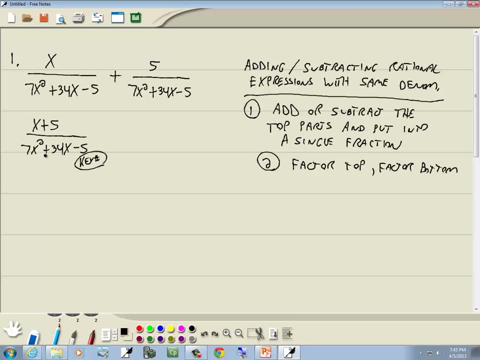 Okay, This is the key number. We got x squared x, no x, and there's a number for our x squared Well, with the key number. we take the number at the beginning times, the number at the end, ignoring signs. 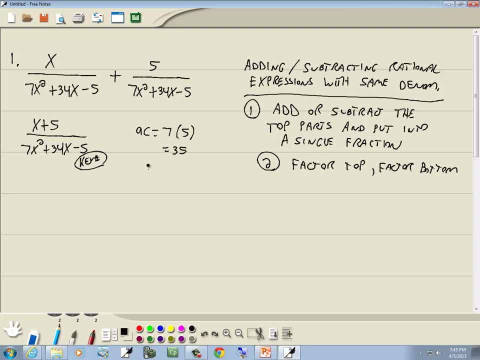 So 7 times 5 gives us 35. And we'll come up with our three columns: Product column, the p column. we write down: all products give us 35.. We got 1 times 35.. We got 2,, 3,, 4, 5 times 7.. 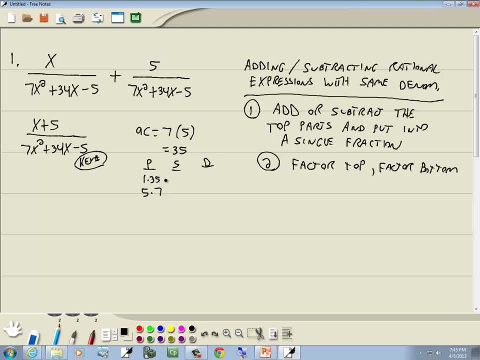 I think that's it, The s column. we add these numbers together: 1 plus 35 is 36.. 5 plus 7 is 12.. The difference column we subtract them: 35 minus 1 is 34.. 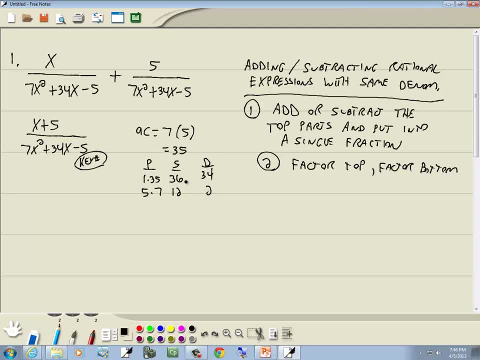 7 minus 5 is 2.. The number we're looking for is the number in our middle term, which is 34, which is right here. So we're going to use 1 and 35.. So we got 7x squared plus 34x minus 5.. 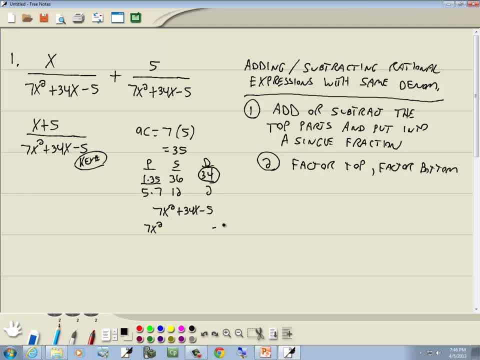 We're going to rewrite our middle term using those two numbers. The larger number in our p column that we're using, which is the 35, is always going to be the same sign as the middle term, which was positive. The number we circled in the difference column, d for different signs means one's positive. 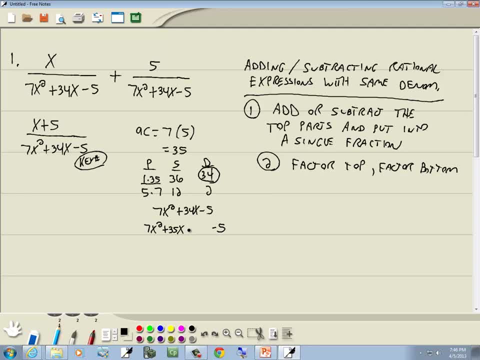 and one's negative. So if the 35 is positive, then the 1 has to be negative, And then we'll factor by grouping The first two terms. The first group, The second group has a 7x in common, and that gives us x plus 5.. 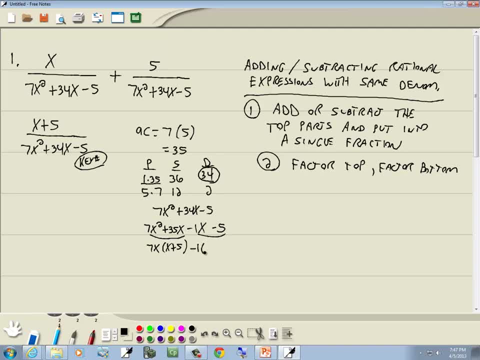 Second group doesn't have anything in common, but my first term's negative, So we'll factor out a negative 1, and that gives us x plus 5.. Now they both have an x plus 5, so I'll factor that out. 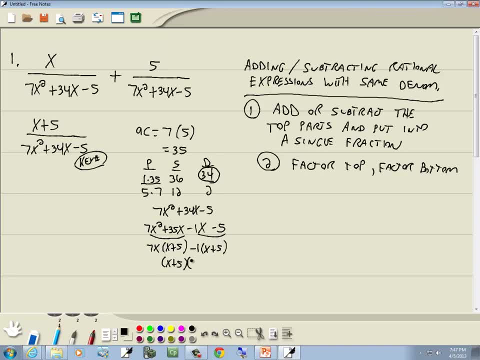 And you basically can cross out the x plus 5s here to see what goes in your second set of parentheses, which would be 7x minus 1.. So this becomes x plus 5.. x plus 5 over x plus 5 times 7x minus 1.. 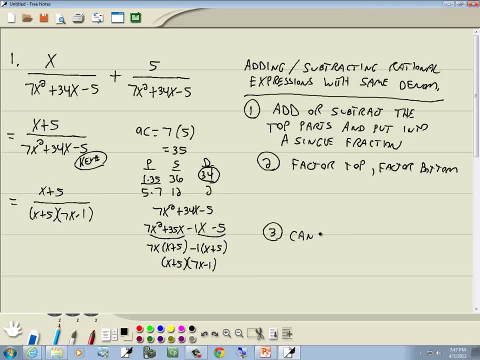 Well, step three: Cancel, if possible. Now notice we have the same item up on top and on the bottom. They both have an x plus 5.. So those x plus 5s are going to cancel And we're left with 1 over 7x minus 1.. 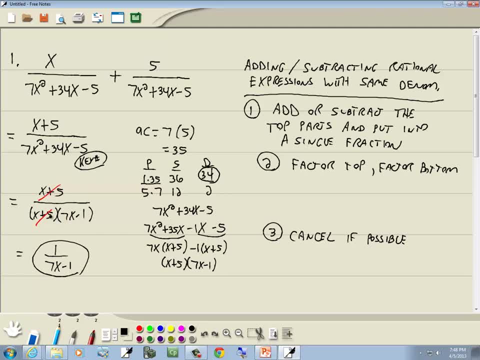 And that's our answer. Now, the reason why we can cancel here is because we got x plus 5 times 7x minus 1.. It's multiplication. You can't cancel up here at our original problem, like the x and the x squared, because you 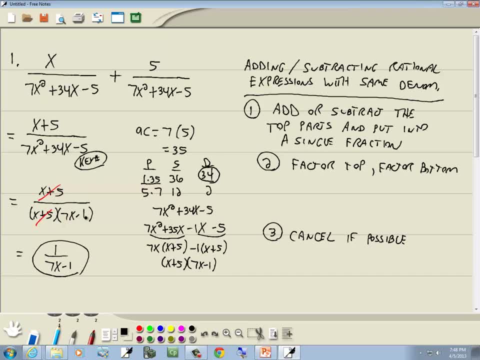 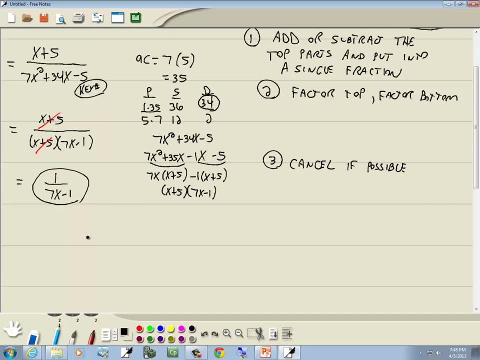 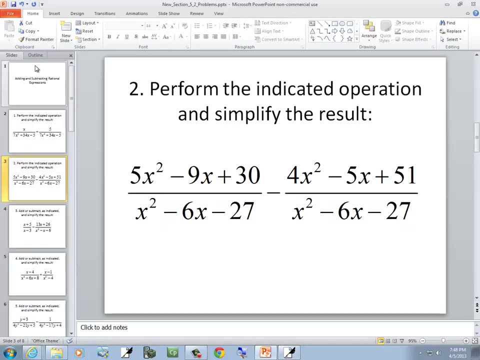 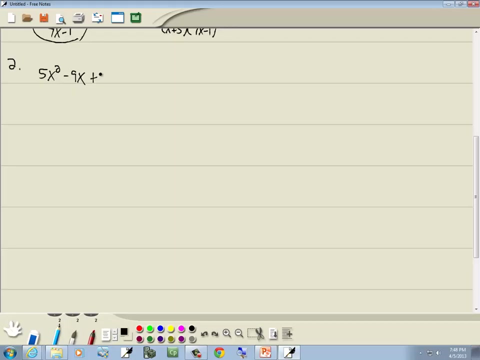 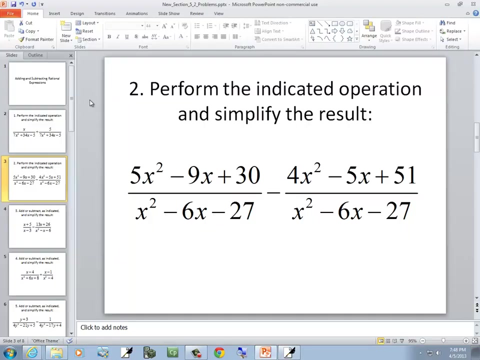 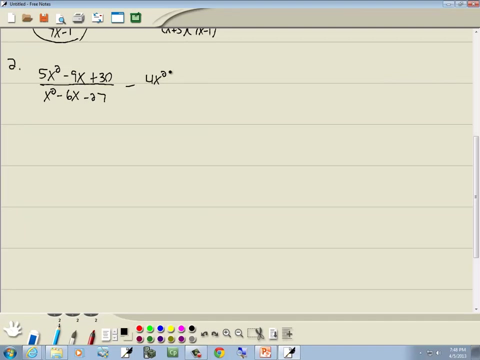 got pluses and minuses in here. You have to have multiplication like this. Let's take a look at another problem. Okay, number two. We've got 5x squared minus 9x plus 30, over x squared, minus 6x minus 27 minus 4x squared. 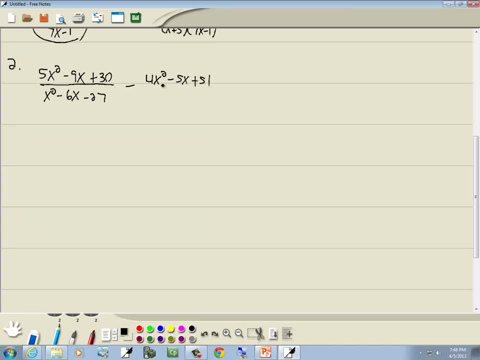 minus 5x Plus 51, all over x squared minus 6x minus 27.. Okay, step one: Add or subtract the top parts. Well, here we have a minus. Now, whenever you have a minus out in front of your fraction, this is going to flip a. 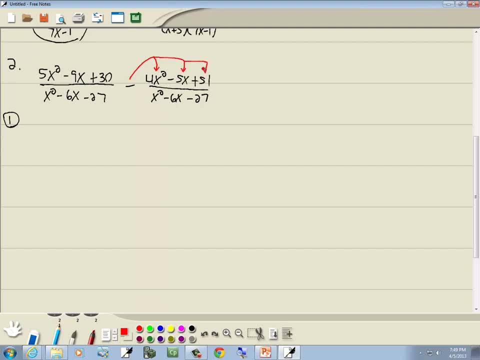 sign of all the terms up on top. So it's going to flip a sign of all those. So this becomes 5x squared minus 9x plus 30 minus 4x squared plus 5x minus 51.. And then denominator stays as is. 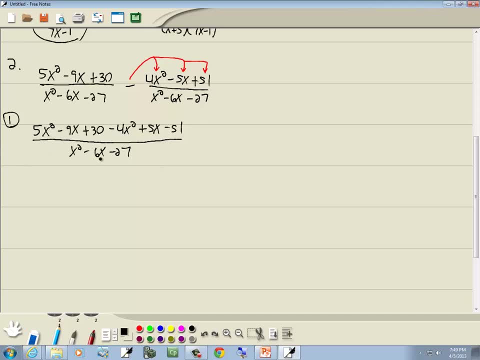 Well, always in math we want to combine together like terms: 5x squared minus 4x squared gives us x squared Negative. 9x plus 5x gives us negative 4x 30 minus 51 is negative 21 over x squared minus 6x minus 27.. 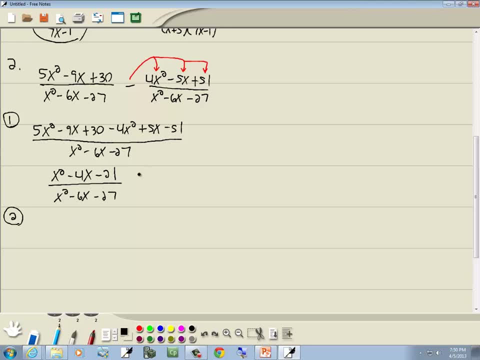 Step two Factor the top factor, the bottom. Both of these are the PSD method. Let's look at the top part first. We got x squared, x, no x. there's no number in front of the x squared. That's what tells us PSD. 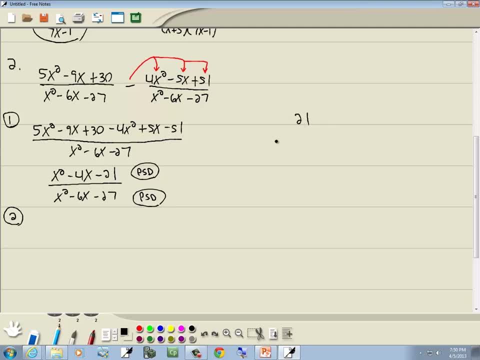 We take the number at the end, the 21,, ignoring signs, and we're going to come up with our three columns, Our p column. We'll write down all products give us 21.. We got 1 times 21,, 3 times 7.. 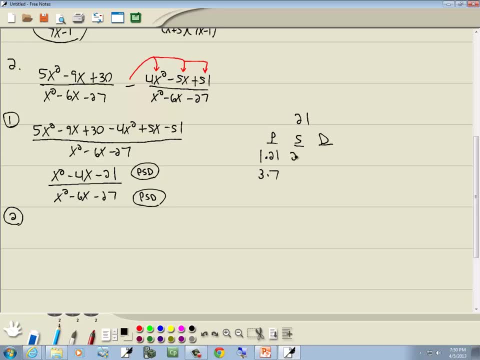 I think that's it. Sum column We add these together: 1 plus 21 is 22.. 3 plus 7 is 10.. The difference column we subtract them: 21 minus 1 is 20.. 7 minus 3 is 4.. 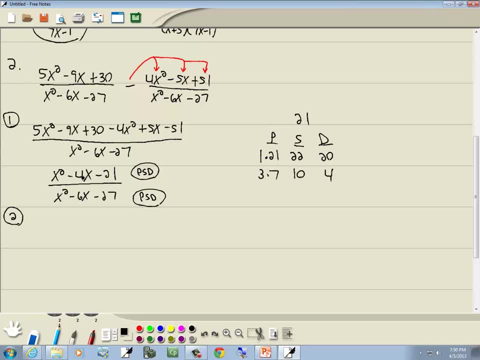 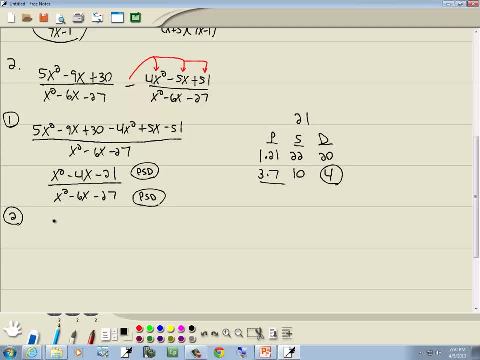 We're going to subtract it. This is 4,, which is right here, so we're going to use 3 and 7.. Now our larger number that we're using in the p column, which is 7, will always be the. 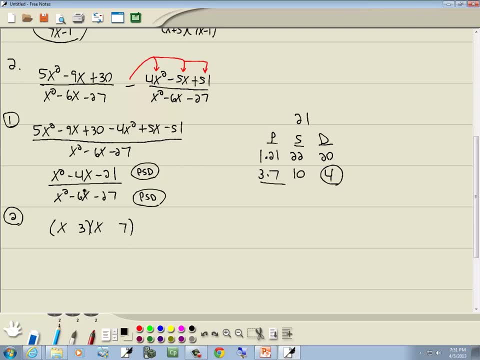 same sign as the middle term. We had a negative 4x, so the middle term is negative, So this is negative, The number we circled in the difference column d for different signs. So if this one is negative then the other one has to be positive. 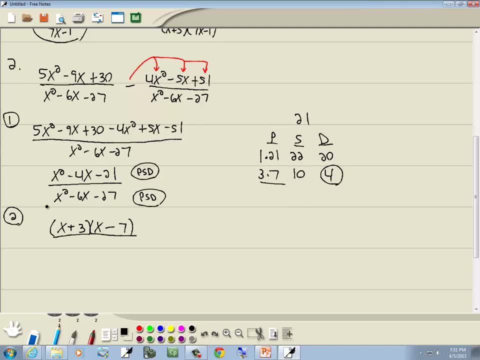 Let's look at the bottom one now. PST again, because it's x squared, x no, x, no number in front of the x squared. Take the number at the end, 27,, and we'll come up with our three columns. 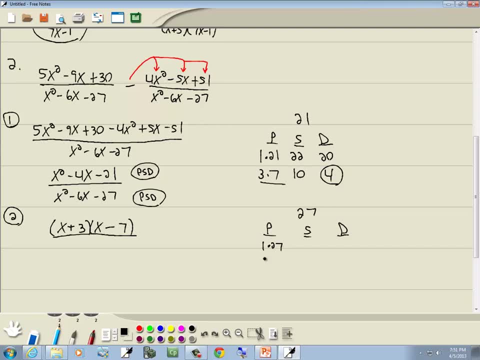 We'll write down all products: give us 27.. We got 1 times 27,, 3 times 9.. The s column: we add them together: 1 plus 27 is 28,, 3 plus 9 is 12.. 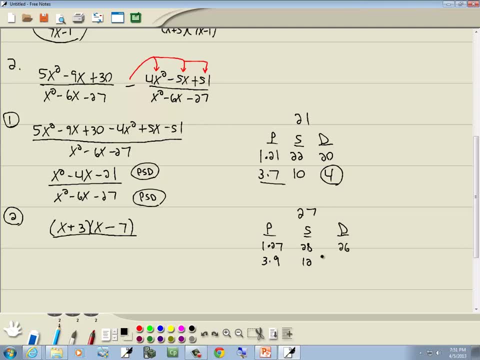 Difference column. we subtract them: 27 minus 1 is 26.. 9 minus 3 is 4.. 3 is 3.. I seem to. oh, I can't subtract, I better go to bed. 9 minus 3 is 6.. 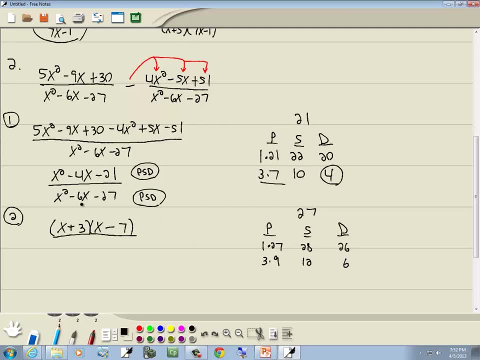 Okay, the number we're looking for is the number in our middle term, which is 6,, which is right here. So we're going to use 3 and 9.. Now our larger number in the p column, which is a 9,, will always be the same sign as the. 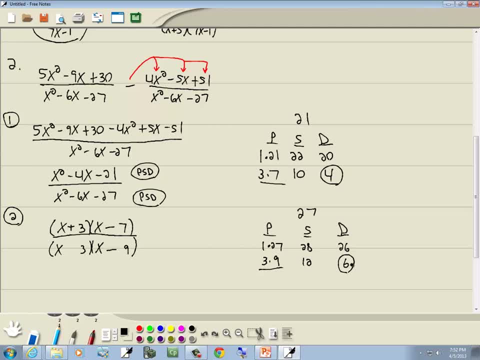 middle term, which was negative. The number I circled in the difference column d for different signs means one's positive, one's negative. So if this one's negative, then the other one has to be positive. Step 3,: cancel if possible. 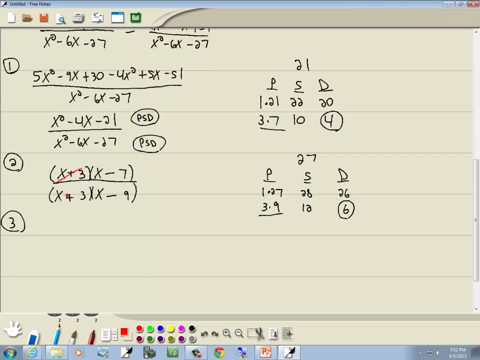 Well, I notice that the top and the bottom both have an x plus 3.. So those are going to cancel And we're left with x minus 7 over x minus 9.. Now the x's can't cancel here. Now the x's can't cancel here. 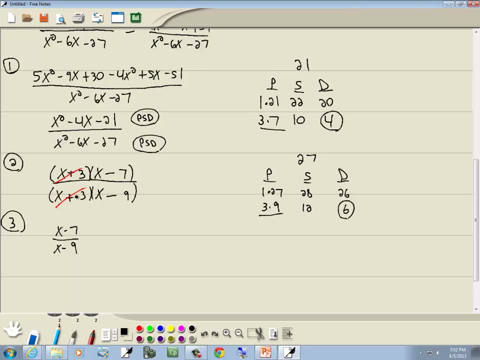 This is x minus 7.. It has to be multiplication for you to be able to cancel. See how this was x plus 3 times x minus 7, and this was x plus 3 times x minus 9.. That's why we could cancel, because those were multiplication. 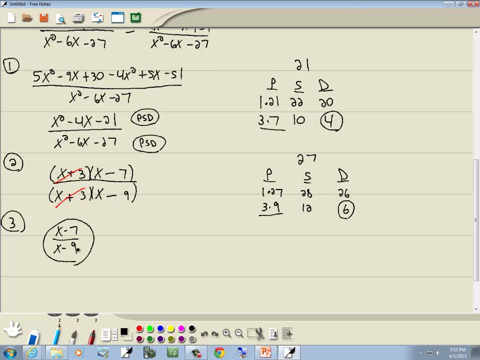 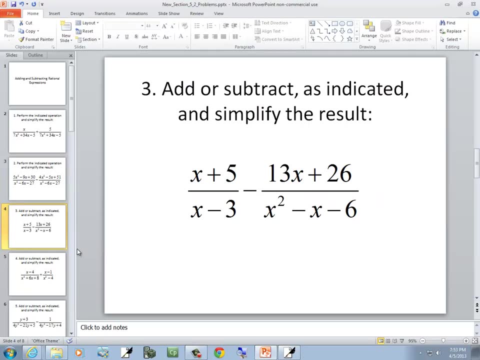 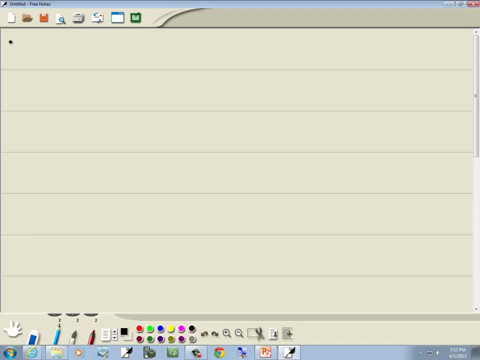 So that's our answer. Now the next problem gets into different denominators. So your denominators aren't the same. So let's take a look at that. We have x plus 5 over x minus 3 minus 13x plus 26.. 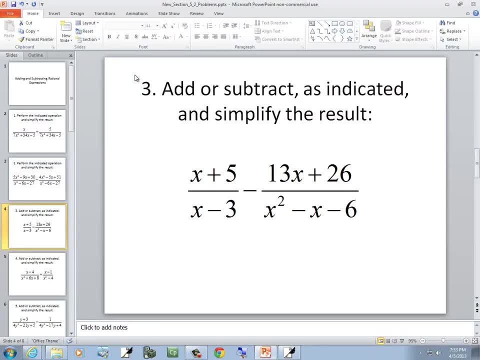 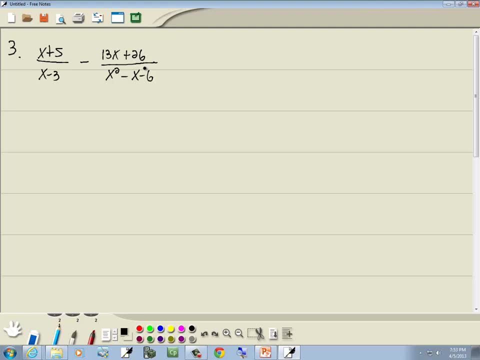 And then we get x squared minus x minus 6.. This one actually has a little bit of a shift. It's a little bit of a shift, It's a shortcut that I'm going to ignore. I will mention it here, But this is going to be adding slash subtracting rational expressions with different denominators. 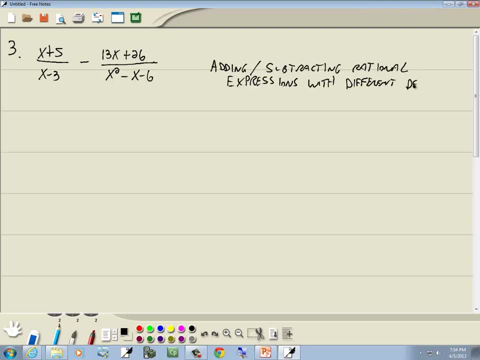 If you can see that, Let me read my writing. So our denominators are different. Well, step one: Factor all the denominators. So factor all the denominators. Now the x minus 3 we can't do anything with, but the other one is a PSD. 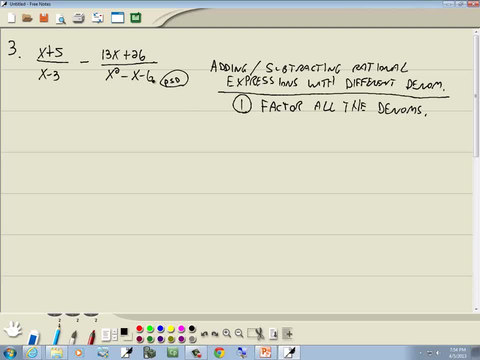 And I didn't hardly leave room here. But we have x squared, x, no x, And there's no number before the x squared. We take the number at the end, which is a 6. And we're going to create our three columns. 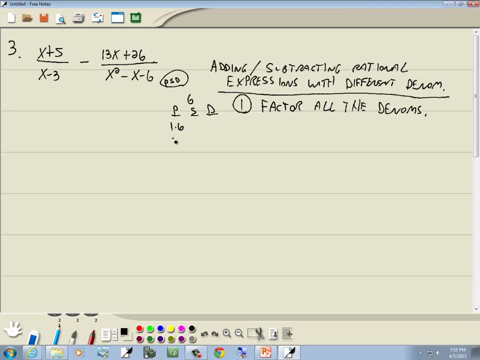 The p column: We write down all products give us 6.. We got 1 times 6,, 2 times 3.. The sum column: We add those together: 1 plus 6 is 7.. 2 plus 3 is 5.. 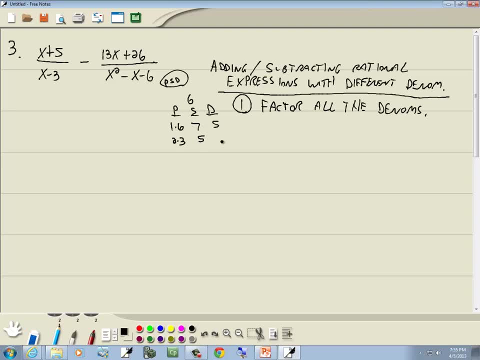 Difference column. Subtract smaller from larger: 6 minus 1 is 5.. 3 minus 2 is 1.. We subtract smaller from larger: 6 minus 1 is 5.. 3 minus 2 is 1.. So we're going to have x here. 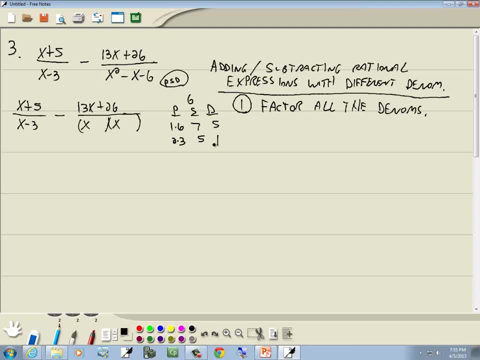 We're going to have x here. The number in the middle is the invisible 1,, which is right. here We're going to use 2 and 3.. Now, our larger number that we're using, which is a 3, is always going to be same. 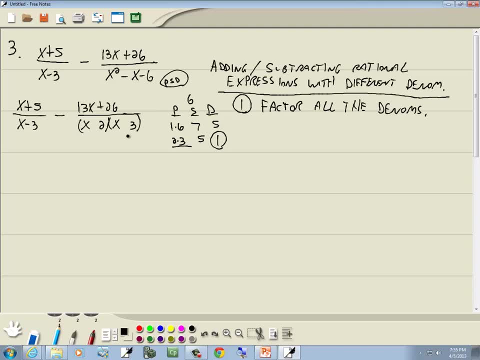 sign as the middle term. Well, middle term was a negative x, 5. be a negative: 3. Number always circles in the difference column D for different signs. So if this is negative, the other one has to be positive. Now, the shortcut on this one is: if you're good at 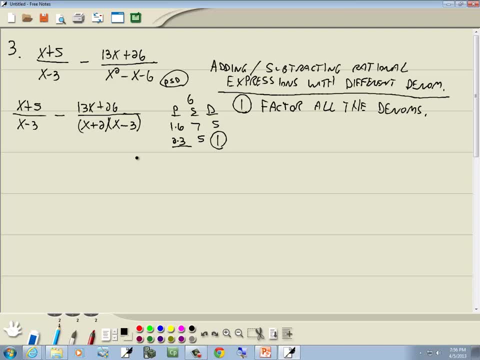 factoring. If you see that you can factor the top and factor the bottom and something would cancel, go ahead and do that Like up on top. notice how these both have a 13 in common. I can factor that out and that gives me an x 13 times x plus 2 and then the x plus 2s would cancel Again. I'm going. 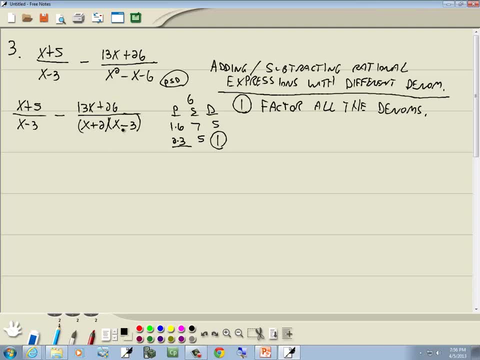 to ignore that Typically people in intermediate algebra aren't that great at factoring. yet They get there after this chapter. But let me let me continue on with this. Step two: Figure out the LCD least commons Denominator, Assuming I can spell So least common denominator And rewrite each fraction. 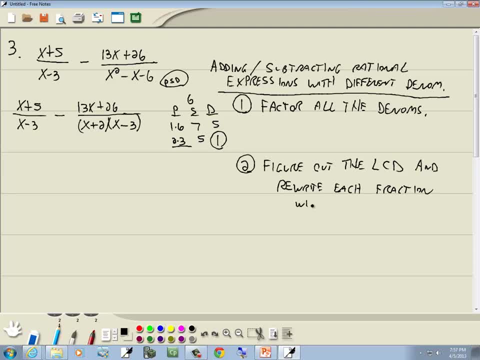 Rewrite each fraction with that denominator. Okay, Let's start off with our first factor, The x minus 3.. Now the question we're going to be asking is: we're looking for the greatest number of x minus 3s in any single denominator. Again, we're. 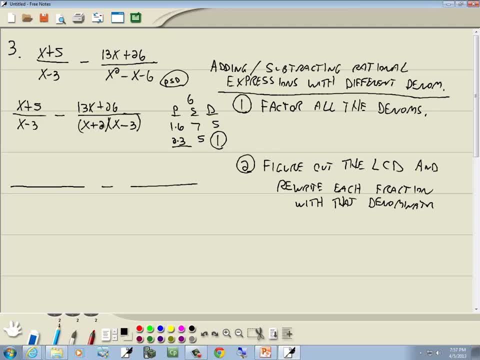 looking for the greatest number of x minus 3s in a single denominator. There's one here and there's one here. So the greatest number of x minus 3s in a single denominator is 1.. Now go to my next factor, the x plus 2.. 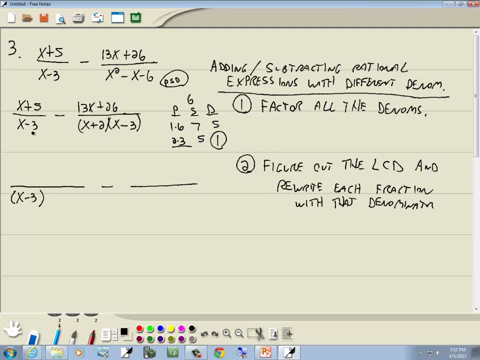 And I'm looking for the greatest number of X plus 2s in a single denominator. There's none here, There's one here. So the greatest number of x plus 2s in a single denominator is 1.. Now, the answer to that will almost always be 1.. So that's our LCD. 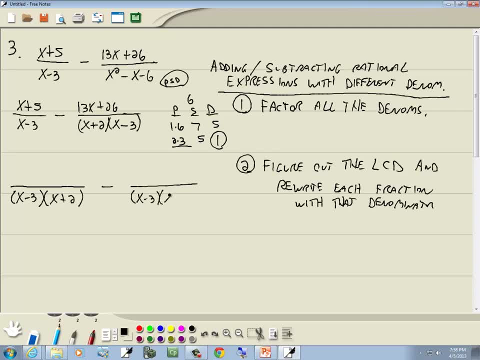 well, after we figure out the LCD, we want to rewrite each fraction with that denominator. Now our second factor for tags. We'll take our of and divide by 10.. Well, the fraction already had that denominator, so it stays as is. So this is 13x plus 26.. Now, if we look at 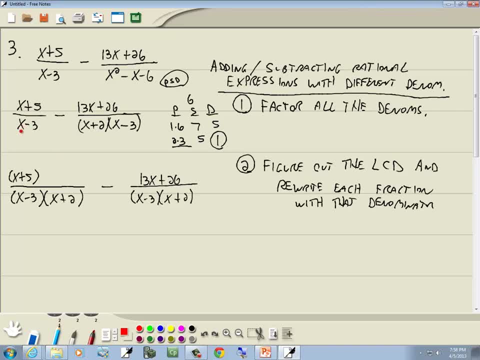 our first fraction, first denominator, we had an x minus 3, the x minus 3 is still there. The new item I put downstairs is the x plus 2.. So whatever new item you put down here you have to put up on top. Now the mathematical principle behind that is: whatever you multiply by the bottom. 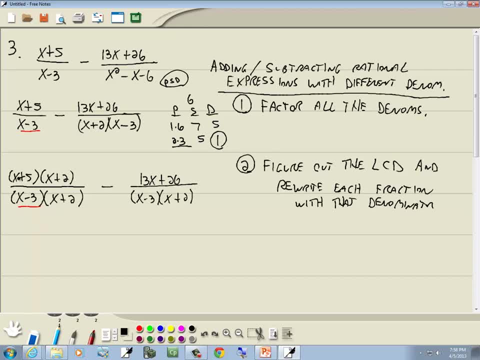 you have to multiply by the top. Well, I'm going to multiply these together: x times x is x. squared x times 2 is 2x, 5 times x is 5x and 5 times 2 is 10.. And the denominator stays the same. 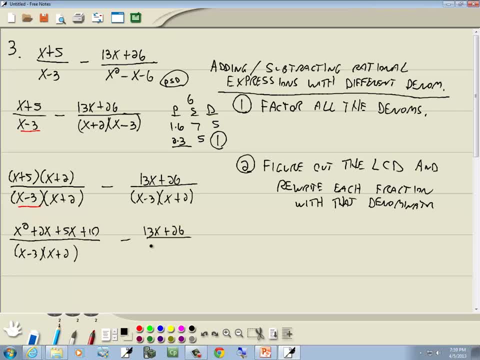 Minus 13x plus 26, over x minus 3 times x plus 2.. Now you need to remember that the denominator stays the same. Now you need to remember that the denominator stays the same. Now you need to remember that the denominator stays the same. 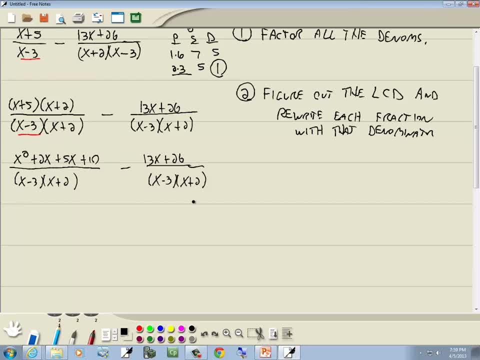 So you never get rid of the parentheses down in the denominator because you're actually hoping they'll cancel away later on. We can still combine these together: 2x plus 5x is 7x, So we've got x squared plus 7x plus 10. 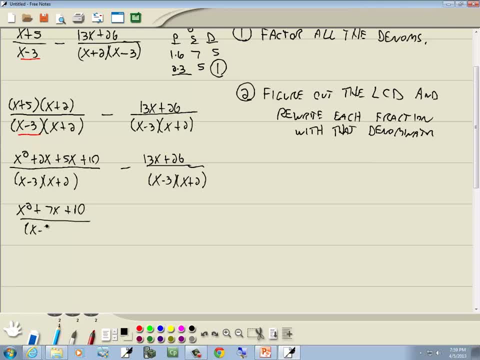 over x minus 3 times x plus 2 minus 13x plus 26 over x minus 3 times x plus 2.. Now you probably notice at this point that they have the same denominators. So this goes back to the steps we just looked at. 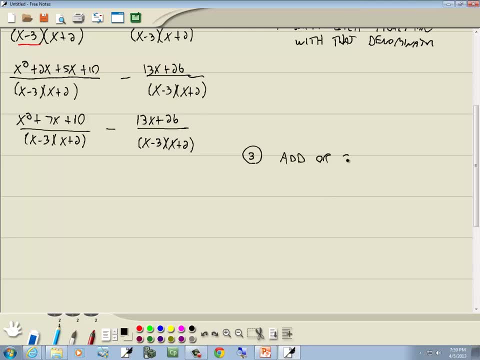 We're going to add or subtract the top parts And put into a single fraction. Now remember: if you have a negative, a minus, out in front of your fraction, it has to flip a sign of all the terms up on top. 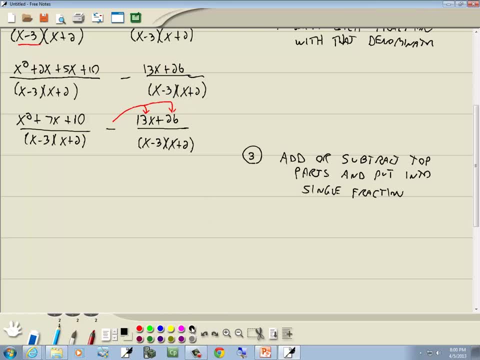 So we're going to flip a sign of 13x and the 26. So this becomes x squared plus 7x plus 10 minus 13x minus 26.. So this becomes x squared plus 7x plus 10 minus 13x minus 26.. 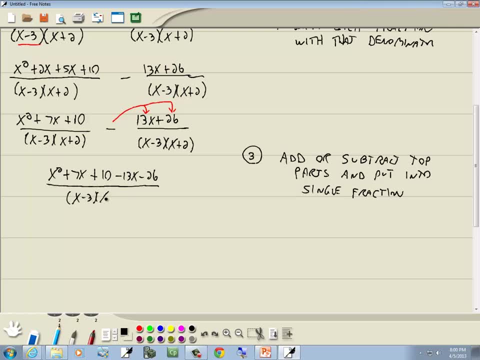 And our denominator stays the same. And our denominator stays the same: Step 16.. Well, no matter where you are in math, combine together like terms. Well, no matter where you are in math, combine together like terms. We've got x squared: 7x minus 13x gives us negative 6x. 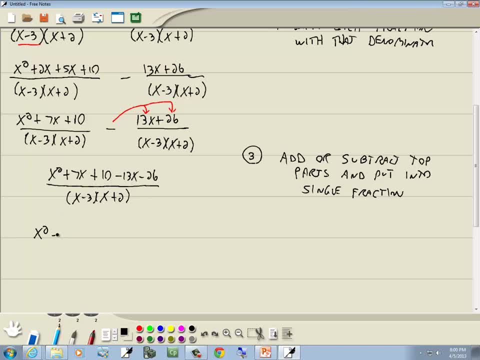 We've got x squared: 7x minus 13x gives us negative. 6x, 10 minus 26 gives us negative 16.. The denominator stays as is. The denominator stays as is Step 4.. Factor the top and factor the bottom. 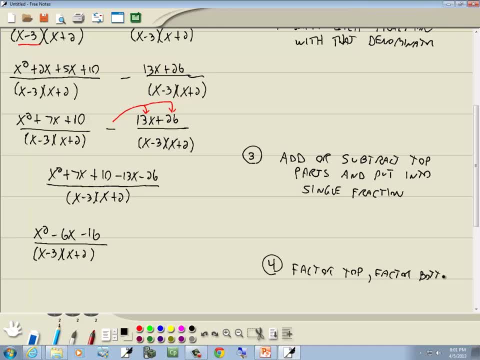 Back to the top and back to the bottom. So factor the numerator and factor the denominator. Therefore it becomes 10 minus 26 plus 9 times x minus 6 x minus 26 is $12.. So it It remains the same denominator. Well, the bottom part's already factored. So unless you actually multiply these, 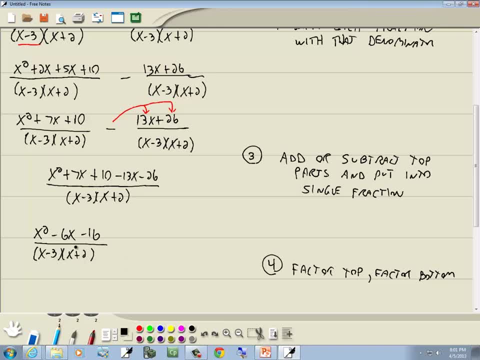 together, which you shouldn't never get rid of the parentheses in the denominator. unless you multiply those together, you shouldn't have to factor the bottom part. The top part, though, is going to be the PSD. We have x squared, x, no, x, no number in front of the x squared. 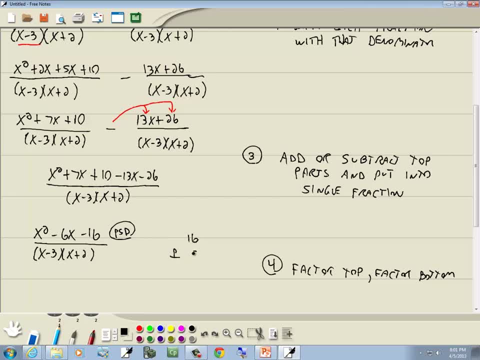 Take the number at the end, which is 16.. We ignore signs. We handle that later on And we'll come up with our three columns. We write down all products. give us 16.. We got 1 times 16,, 2 times 8,, 4 times. 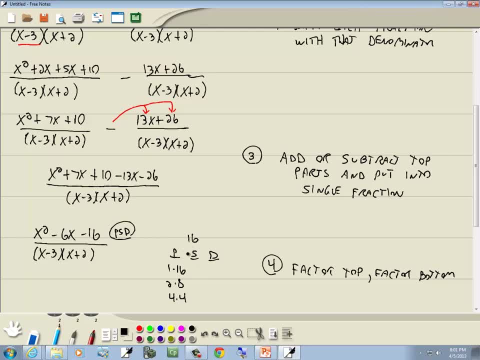 4. The S column: we're going to add those together: 1 plus 16 is 17.. 2 plus 8 is 10.. 4 plus 4 is 8.. The difference column we'll subtract smaller from larger: 16 minus 1 is 15.. 8 minus 2 is 6.. 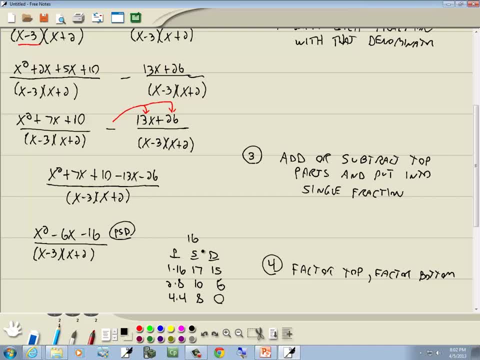 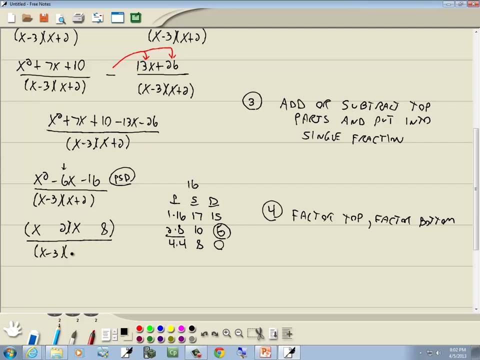 4 minus 4 is 0.. Now the number we're looking for is a number in our middle term, which is a 6, which is right here. So we're going to use 2 and 8.. Okay, The two numbers we're going to use- 2 and 8, the larger number that we're using. 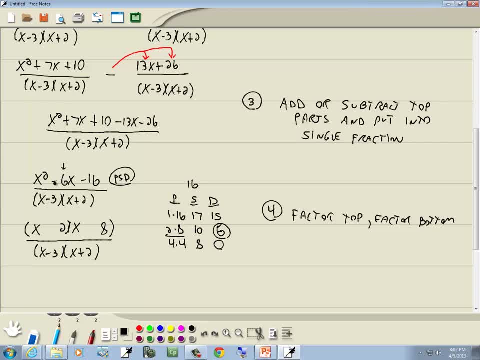 which is the 8, will always be the same sign as the middle term. The middle term is a negative 6x, so it's negative. So the 8 will be negative, The number we circled in the difference column d for different signs. So if this one's negative, the other one is positive. 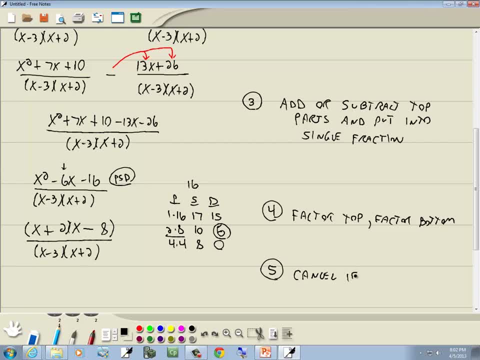 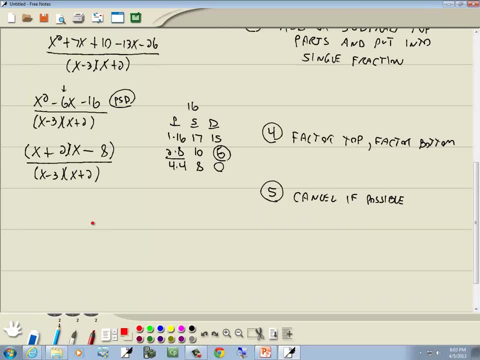 And step 5. Cancel if possible. You can cancel if they're the same. See how we have an x plus 2 here, an x plus 2 here. Those are going to cancel. So we end up with x minus 8 over 8.. 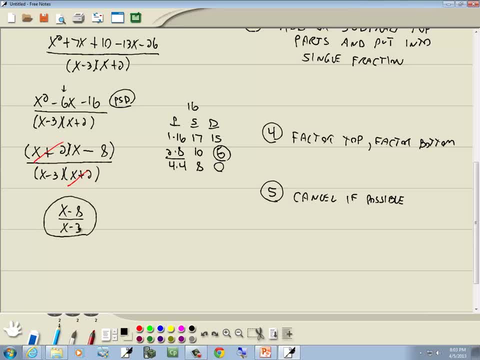 Minus 8 over x minus 3.. And again, we cannot cancel the x's because of the minus. in here Everything has to be multiplication. We'd have to have x times 8 and x times 3 for us to be able. 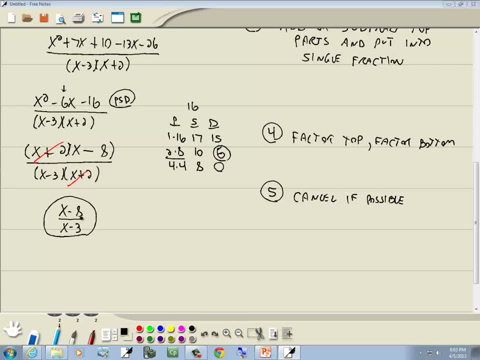 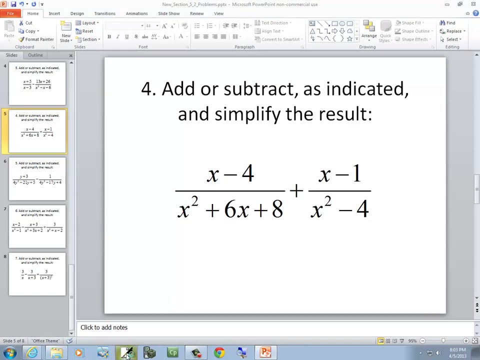 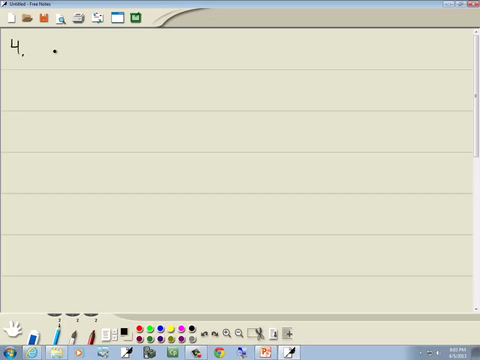 to cancel. Okay, Let's look at this one. Let me start a new page. Oh, Okay, so number 4. We have x minus 4 over x squared, plus 6x plus 8, plus x minus 1 over x squared. 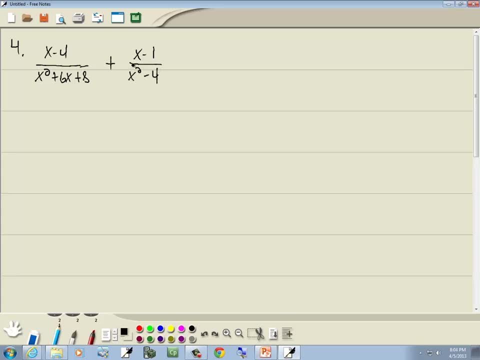 minus 4.. Step 1. Factor our denominators. This one here is the PSD method and this one is the dots Difference: two squares. Let's first look at the x squared plus 6x plus 8. PSD because it's x. 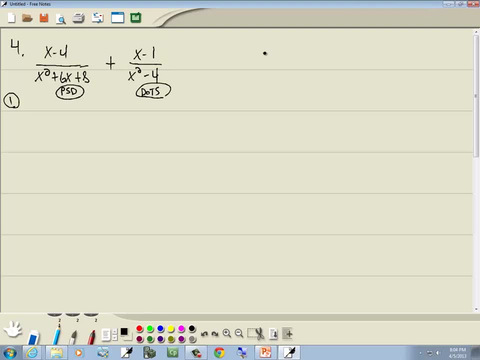 squared x, no, x, no number. in front of the x squared PSD, we take the number at the end, the 8, and we come up with our three columns. P is a product to give us 8.. So we've got 1 times 8, 2. 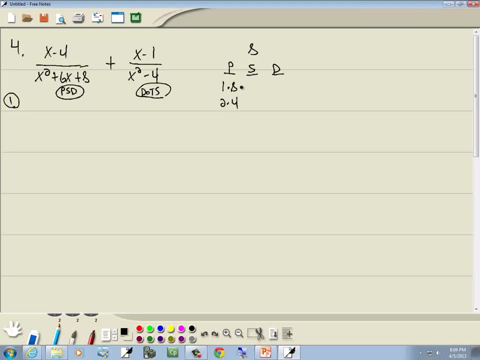 times 4.. The S column: we add those together: 1 plus 8 is 9.. 2 plus 4 is 6.. Difference column: we subtract them Smaller from larger: 8 minus 1 is 7.. 4 minus 2 is 2.. Number we're looking for is the number in our 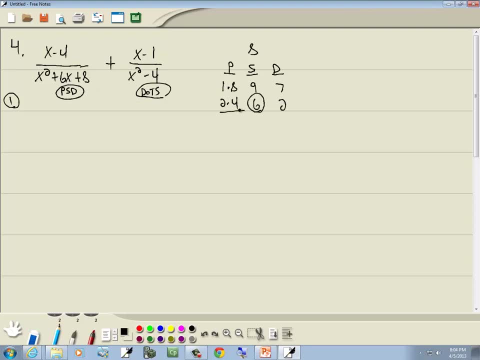 middle term, which is 6.. So we're going to use 2 and 4.. 2 and 4.. Now our larger number that we're using, which is the 4, is always going to be the same sign as the middle term, which is positive, The number I circled in the S column S for 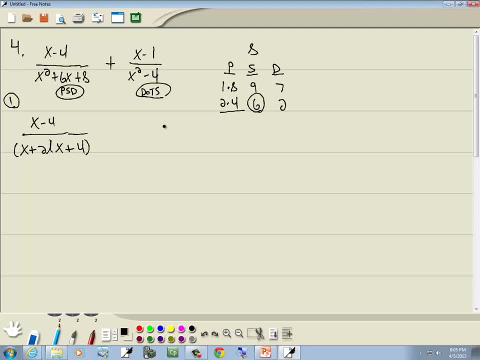 same sign. So if this one's positive, then 2 will be positive. Okay, The x squared minus 4.. Difference: two squares. We try to write it as something squared minus something else squared. You ask yourself what times itself gives you the x squared. Well, 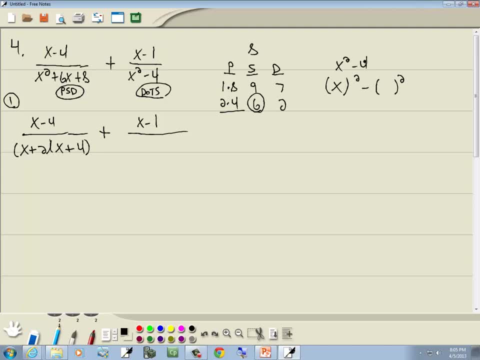 x times x gives you x squared, And you ask yourself what times itself gives you the 4, and 2 times 2 gives you the 4.. Now, if you're able to write it as something squared minus something else squared, you take what's inside your first set of parentheses, you add what's. 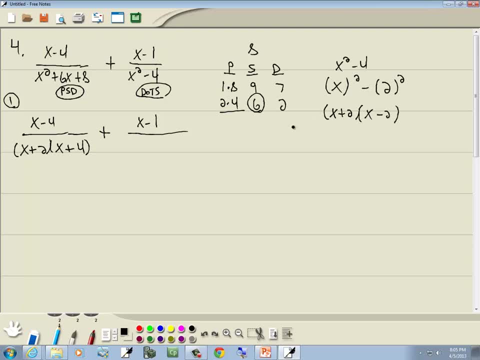 in your last and you take what's inside your first and you subtract what's in your last. So this factors as x plus 2 times x minus 2.. And that's step one. Now step two: Figure out your least common denominator. Let's start there. So our first factor is the x plus 2.. And we're looking. 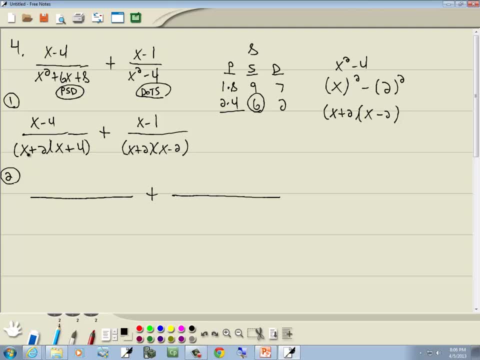 for the greatest number of x plus 2s in a single denominator. There's one here, There's one here. So the greatest number of x plus 2s in a single denominator is 1.. Now again, we're not counting how many there are, We're just looking for the greatest number in a single denominator. 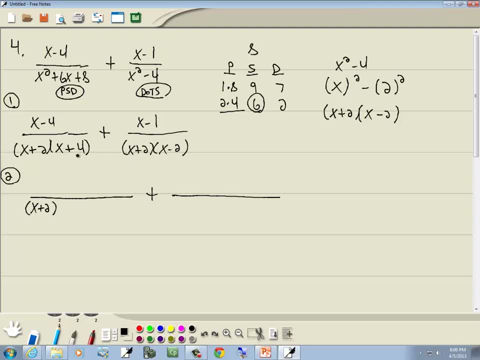 Then I've got my next one, the x plus 4.. I'm looking for the greatest number of x plus 4s in a single denominator. There's one here, There's none here, So the greatest number of x plus 4s. 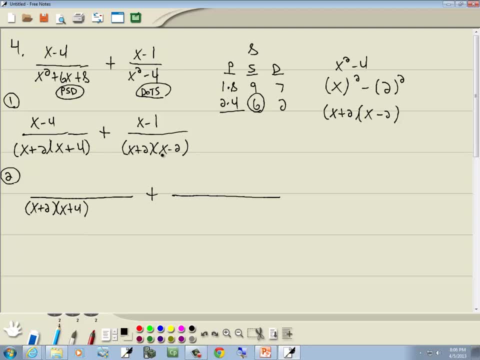 in a single denominator is 1.. And then our last factor, the x minus 2.. I'm looking for the greatest number of x minus 2s in a single denominator. There's none here, There's one here, So we'll. 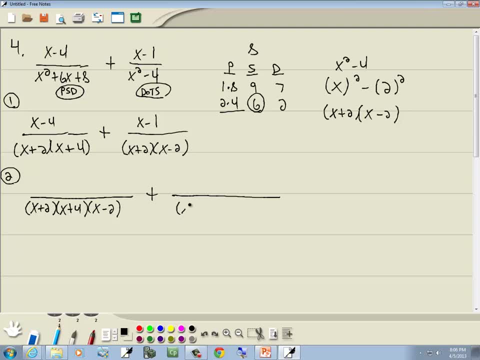 have 1.. So that's our LCD. Now we're going to look at our old fraction and see what new item was put down below. Let me write these down first: x minus 4 and x minus 1.. Looking at our first fraction, we had an. 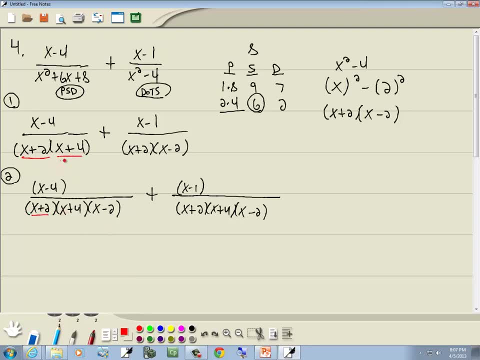 x plus 2.. The x plus 2 is still there. We had an x plus 4.. The x plus 4 is still there. The new item that's downstairs in the denominator is the x minus 2.. So we have to put an x minus 2 up here. 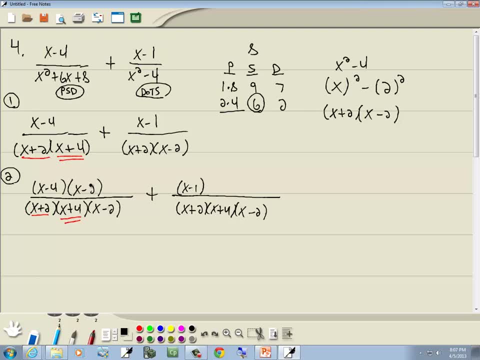 Whatever new item appears down here, you have to put up here Again mathematical rule, and this last time I'll say it: Whatever you multiply by the bottom, you have to multiply by the top. Now, in our second fraction we had an x plus 2.. The x plus 2's still there. We had an. 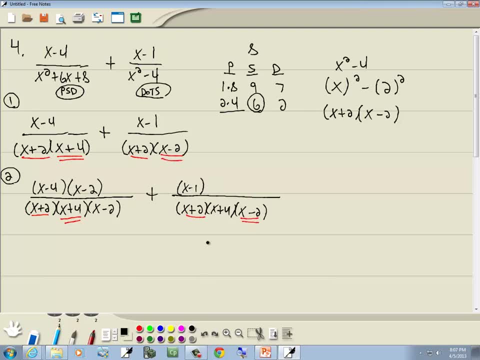 x minus 2.. The x minus 2's still there. The new item down in the denominator is x plus 4.. So we had to put an x plus 4 up here. We're going to get rid off parentheses up on top. combining to the like terms. 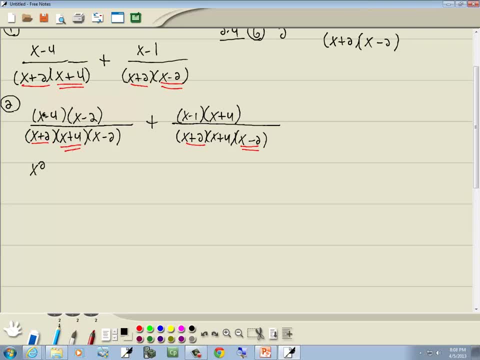 So we got: x times x is x squared, x times negative. 2 is negative, 2x Negative. 4 times x is negative, 4x, As Iあー x and negative. 4 times negative. 2 gives us a positive 8.. 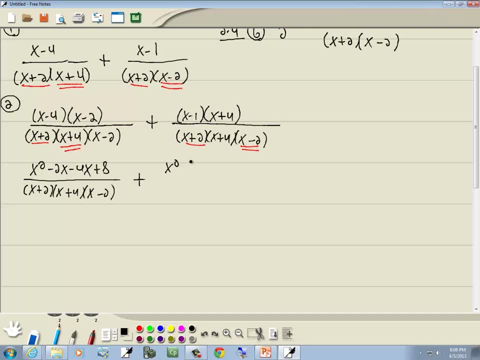 Now over here: x times x is x squared, x times 4 is 4x negative. 1 times x is negative 1x or negative. x negative 1 times 4 is negative 4.. Well, combined together like terms, so we're going to have x squared negative, 2x negative. 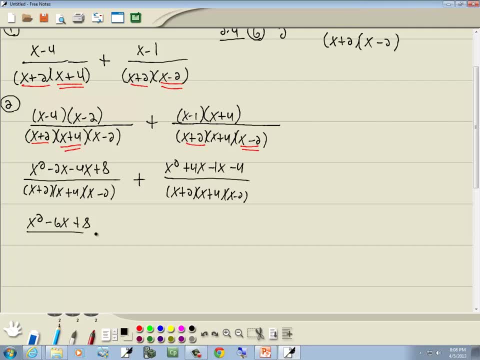 4x is negative, 6x and all the rest of this stays the same. Over here, combined together like terms, we've got 4x minus 1x. that gives us 3x and everything else stays the same. 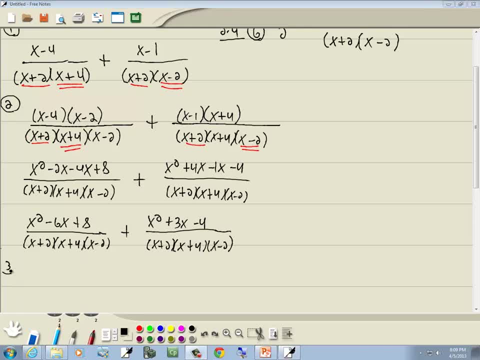 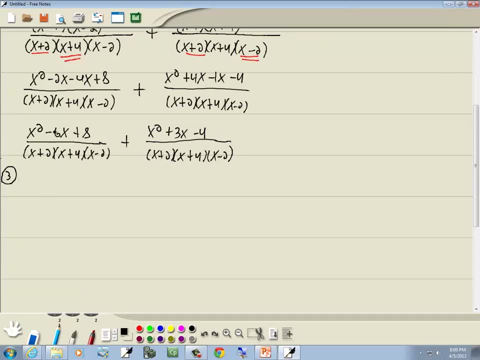 Okay, step three: We want to add or subtract the top parts and merge into a single fraction. So we're going to have x squared minus 6x plus 8 plus x squared plus 3x minus 4, and we're going to have x squared minus 6x plus 8, plus x squared plus 3x minus 4,. 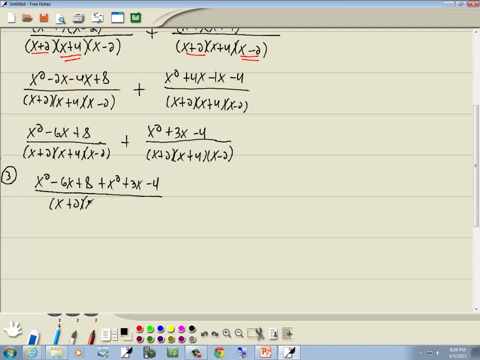 all over our denominator, Well combined together like terms: x squared plus x squared is 2x, squared negative 6x plus 3x is negative 3x and 8 minus 4 gives us 4.. I'm thinking that this doesn't actually factor the top part, because remember our fourth step. 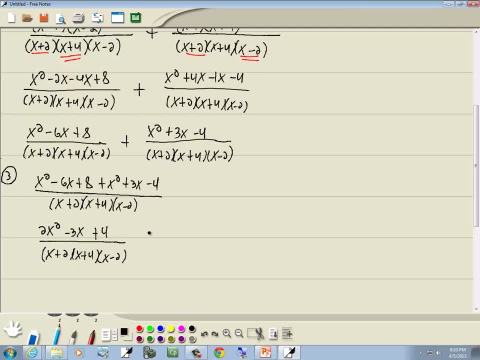 is to factor the top part. We're going to factor the bottom. If it would factor, it's the key number. so let's try that. The reason why it's key numbers is because we have x squared x, no x, and there's a. 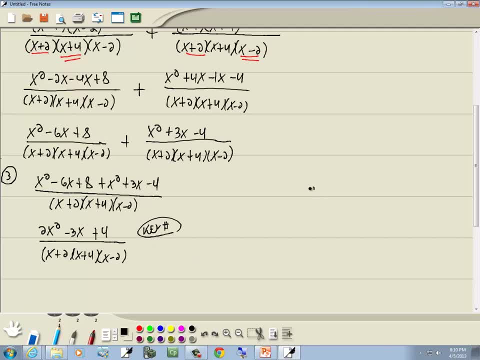 number in front of our x, squared With a key number. we take our number at the beginning, times the number at the end. so we've got 2 times 4, which gives us 8.. We'll write down: all products give us 8, so we've got 1 times 8, 2 times 4.. 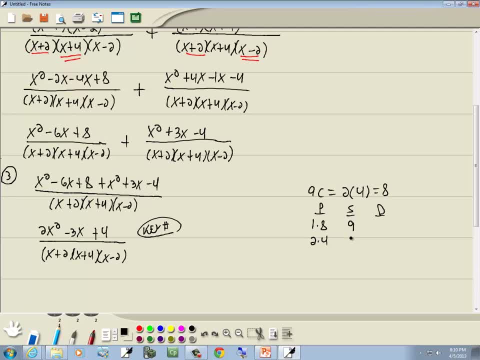 The s column. we add them together: 1 plus 8 is 9.. 2 plus 4 is 6.. The difference column we subtract smaller from larger: 8 minus 1 is 7.. 4 minus 2 is 2.. 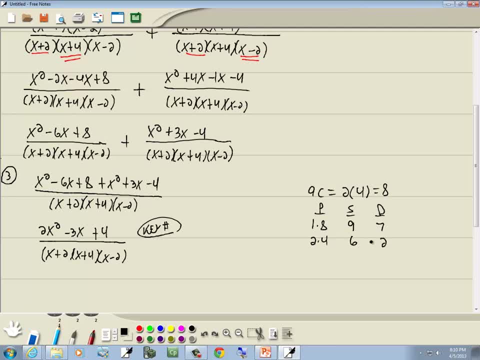 The number we're looking for is the number on our middle term, which is 3, which we don't have. So, assuming I didn't forget any products or added or subtracted incorrectly, this won't factor. And since that won't factor, we obviously can't cancel. so this is our answer, right? 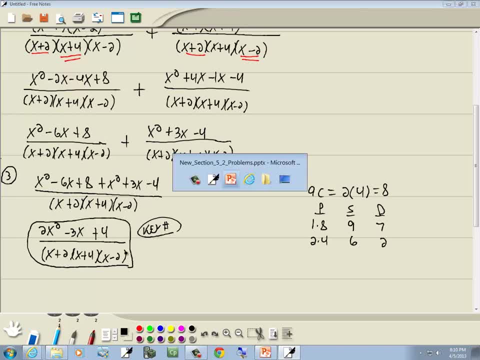 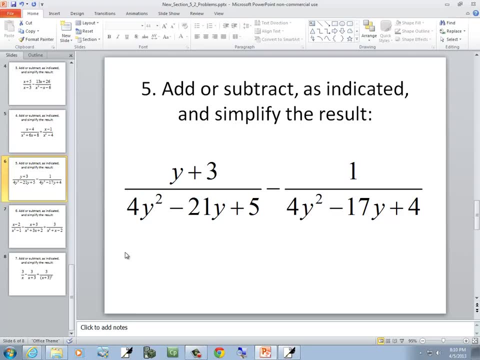 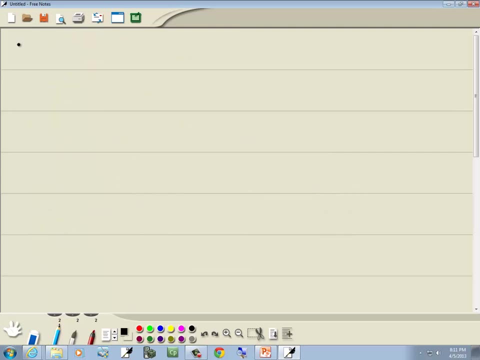 here. Let's take a look at our next problem. Let me grab a drink here. Let's see Number 5.. We have y plus 3 over 4 y squared minus 21y plus 5 minus 1 over 4 y squared plus. 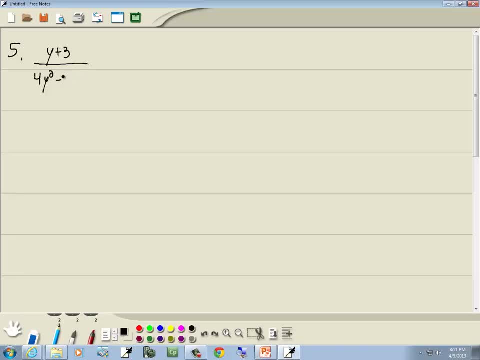 12 y. So we're going to take the new Greek. In the new Greek we were going um動p, which we're going to do ys, squared byando, and we're going to add it to the Greek and we're going to add it to our version saying: 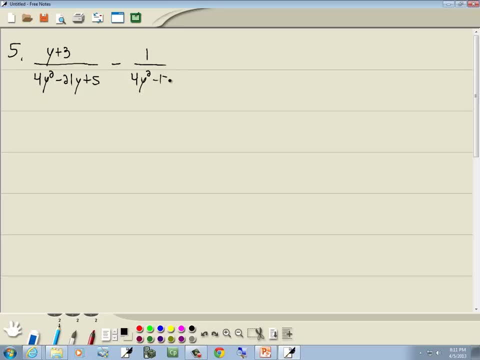 cpc- Whatever- minus 17y plus 4.. First step: factor our denominators. So let's start with this first one. here We've got 4y squared minus 21y plus 5.. This is the key number. 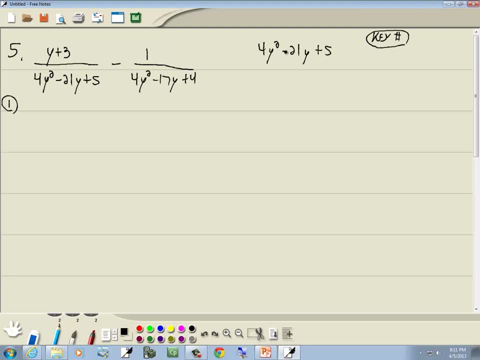 The reason why I know it's a key number is y squared y, no y, and there's a number in front of our y squared, The key number. we take our number at the beginning times the number at the end. So we take 4 times 5, which gives us 20.. 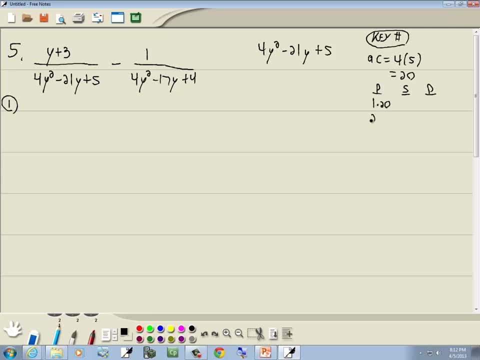 Write down all products give us 20.. We've got 1 times 20,, 2 times 10,, 4 times 5.. The s column add them together: 1 plus 20 is 21,, 2 plus 10 is 12,, 4 plus 5 is 9.. 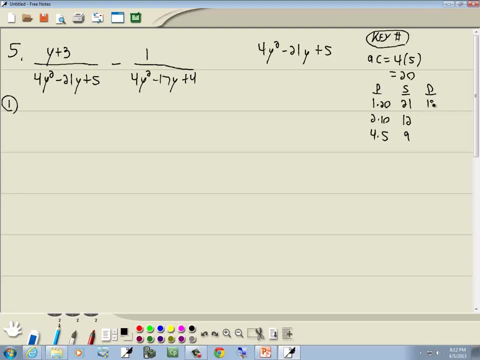 Difference column. subtract them: 20 minus 1 is 19,. 10 minus 2 is 8.. 5 minus 4 is 1.. The number we're looking for is the number in our middle term, which is 21,. 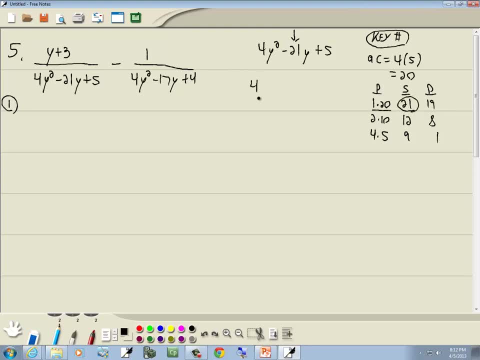 which is right here. so we're going to use 1 and 20.. And remember, we rewrite our middle term using those two numbers. Now the larger number, which is the 20, is always going to be the same sign as the middle term, which is negative. 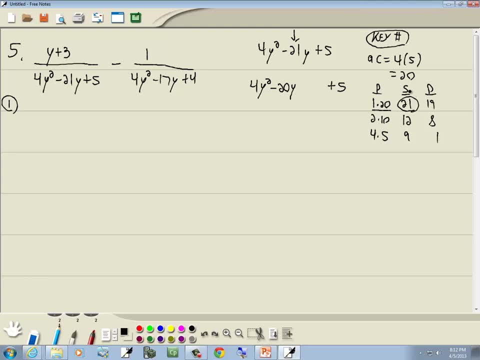 So that's negative 20y, The number I circled in the s column s for same signs. So if the 20 is negative, the 1 has to be negative. So we've got negative 1y Factor by grouping. 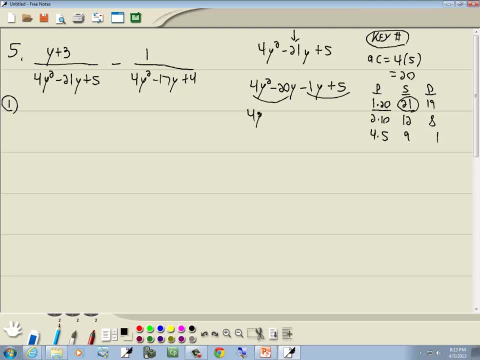 First group, the first two terms have a 4y in common, And that gives us y minus 5.. Second group has nothing in common, but the first term is negative, so I'll factor out a negative 1, and that gives us y minus 5.. 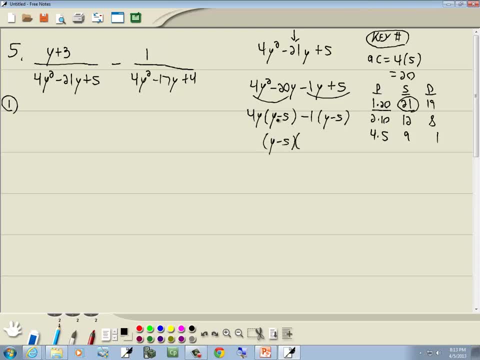 Now they both have a y minus 5, so I'll factor that out And you can cross out the y minus 5s to see what goes in your second set of parentheses, which would be the 4y minus 1.. So that's the first term. 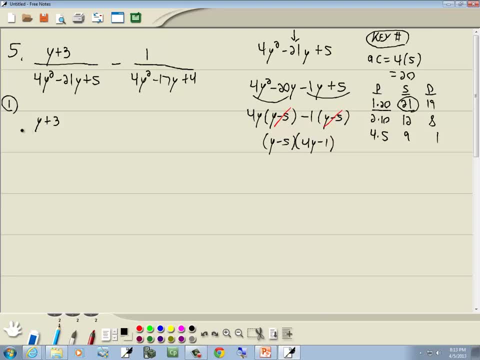 So this first fraction becomes y plus 3 over y minus 5 times 4y minus 1.. Well, let's look at our second denominator. We've got 4y squared minus 17y plus 4.. This is again the key number. 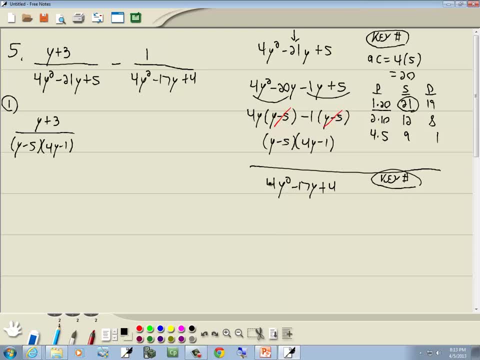 Because we have y squared, y, no y, and there's a number in front of our y squared. Now we'll take our number at the beginning, times the number at the end. So we've got 4 times 4, which gives us 16.. 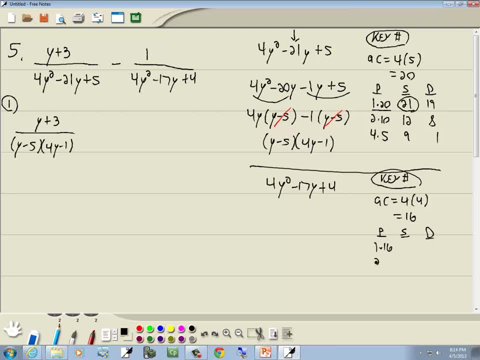 Write down all the products give us 16.. We've got 1 times 16,, 2 times 8,, 4 times 4.. S column: we want to add those together: 1 plus 16 is 17,. 2 plus 8 is 10,, 4 plus 4 is 8.. 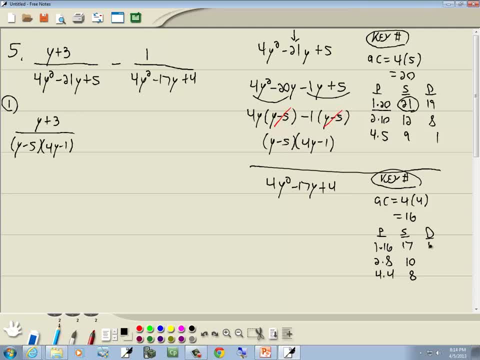 Difference column. we want to subtract smaller from larger: 16 minus 1 is 15,. 8 minus 2 is 6.. 4 minus 4 is 0.. The number we're looking for is always the number in our middle term, which is 17.. 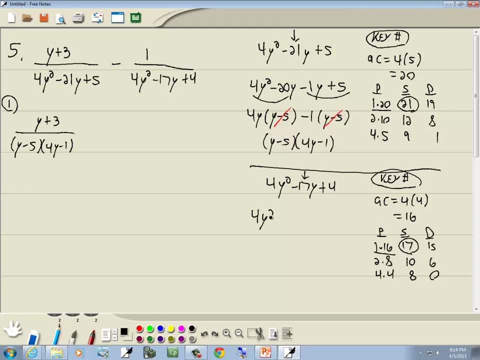 So we're going to use 1 and 16.. And again, what we do with that is we rewrite our middle term using those two numbers. Our larger number, which is a 16, will be the same sign as the middle term, which was negative. 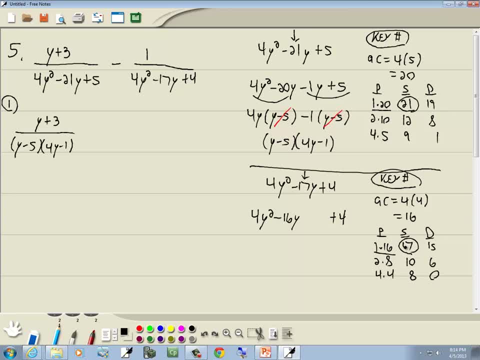 The number I circled is in the S column, which means there's S for same signs. So if 16 is negative, then the 1 will be negative. Then I'll factor by grouping. First group has a 4y in common and that gives us y minus 4.. 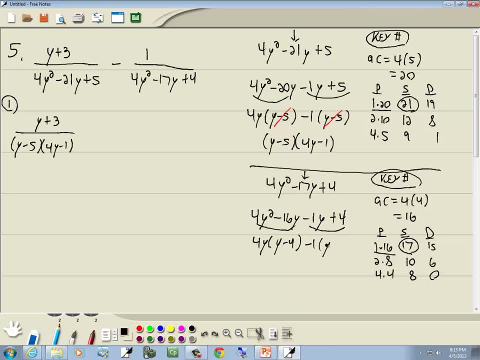 Second group, first term is negative, so I'll factor out negative 1, and that gives us y minus 4.. Now they both have a y minus 4.. And again you can cross out the y minus 4s to see what goes in your second set of parentheses. 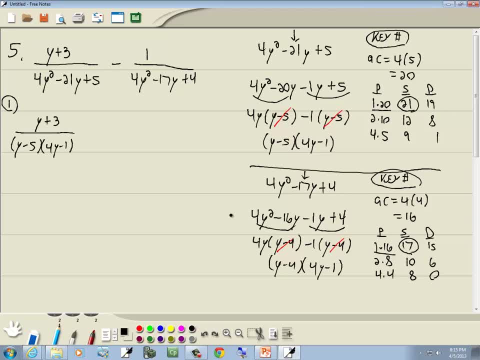 which would be 4y minus 1.. So this second fraction factors as y minus 4 times 4y minus 1.. And now, step one, Step two: Figure out your LCD, your least common denominator. Let's start there. 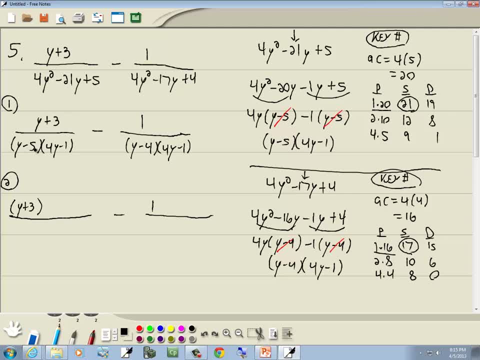 I look at my first factor, the y minus 5.. And I know you get tired of hearing me say this, but I just want to really understand, Emphasize it: We're looking for the greatest number of y minus 5s in a single denominator. 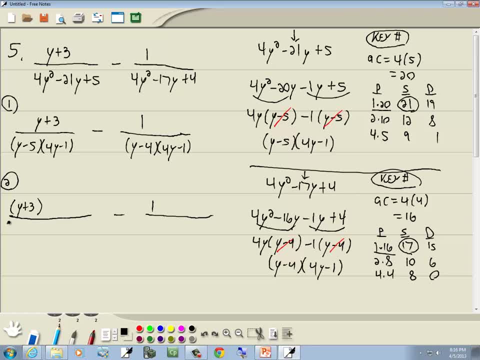 Well, there's 1 here, There's none here, So greatest number of y minus 5s in a single denominator is 1.. Then I go to my 4y minus 1.. And we're looking for the greatest number of 4y minus 1s in a single denominator. 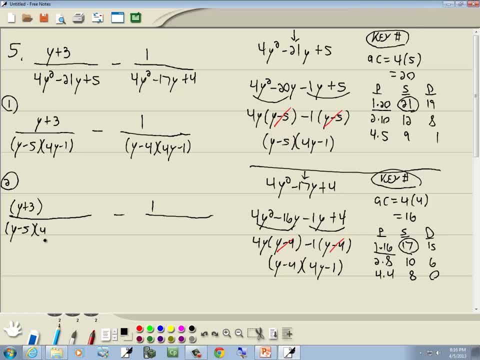 There's 1 here, There's 1 here. So greatest number of 4y minus 1s is 1.. Then we'll go to our next factor, the y minus 4.. I'm looking for the greatest number of y minus 4's in a single denominator. 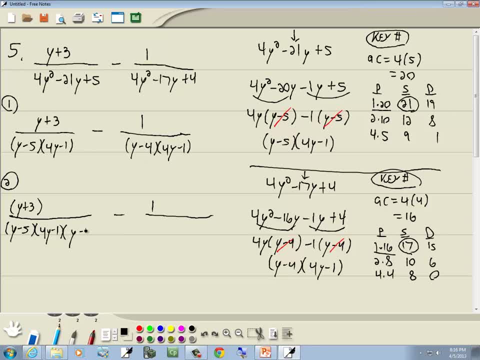 There's none here, There's one here. So greatest number of y minus 4's is 1.. With the exception, I think, of the last problem. Yeah, last problem. The answer will always be 1 on these, And you won't want to cross many in a homework where the answer is 2 or 3.. 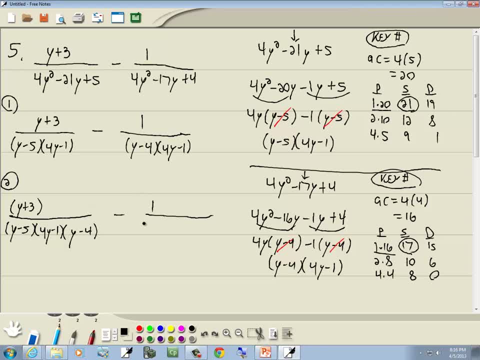 They just get too hideous. So that's our LCD. Okay, Well, we want to figure out. we're rewriting each fraction with that new denominator, So we have to figure out what's changed Here. we had a y minus 5.. 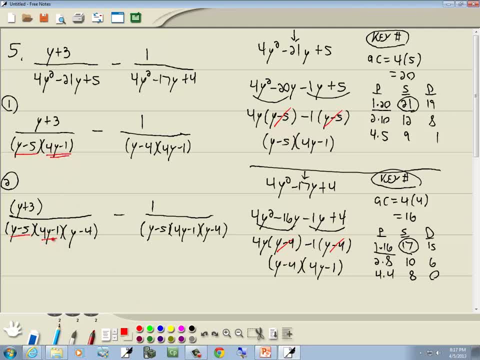 A y minus 5 is still there. 4y minus 1.. 4y minus 1 is still there. The new item down below is the y minus 4.. So we have to put that up on top Now. over in our second fraction we had y minus 4.. 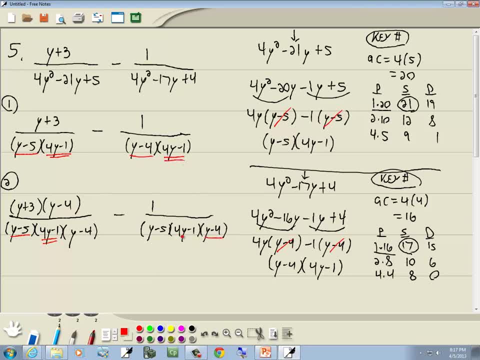 y minus 4 is still there. 4y minus 1 is still there. The new item down below is the y minus 4.. y minus 5.. So I have to put a y minus 5 up on top. Well, I want to multiply those together. 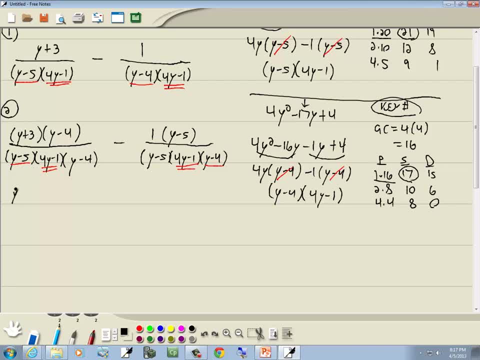 Leave the bottom part alone. y times y is y squared. y times negative: 4 is negative. 4y 3 times y is 3y. 3 times negative, 4 is negative 12.. And over here, 1 times y minus 5 is just y minus 5.. 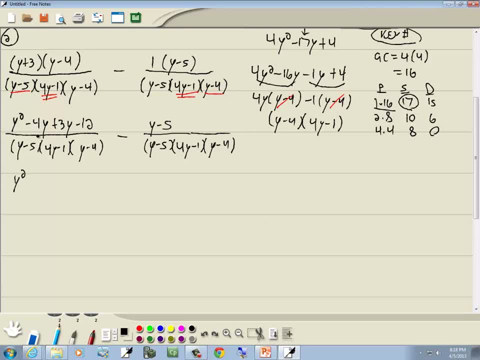 Well, combine the other like terms here. So we're going to have y squared negative 4y plus 3y is negative 1y or negative y minus 12.. Over this Minus y minus 5. over y minus 5, 4y minus 1, y minus 4.. 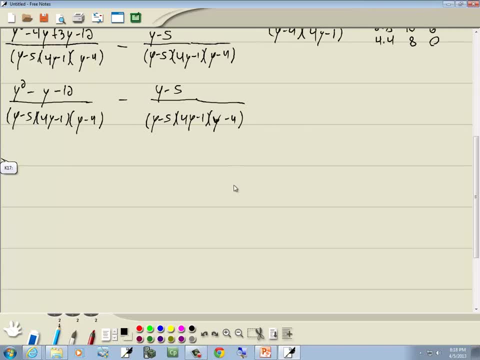 Okay, Step 3.. They have the same denominator now. So we want to add or subtract the top parts and merge into a single fraction. Remember: a negative out in front of your fraction flips the sign of everything up on top. So this negative is going to flip the sign of the y and the negative 5.. 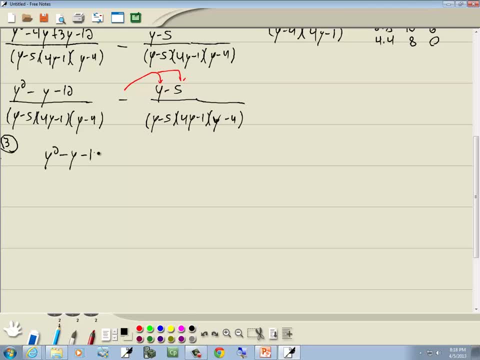 So we have y squared minus y minus 12, minus y plus 5, all over, y minus 5,, 4y minus 1, y minus 4.. Combine together like terms Negative y negative. y is negative, 2y Negative. 12 plus 5 gives us negative 7.. 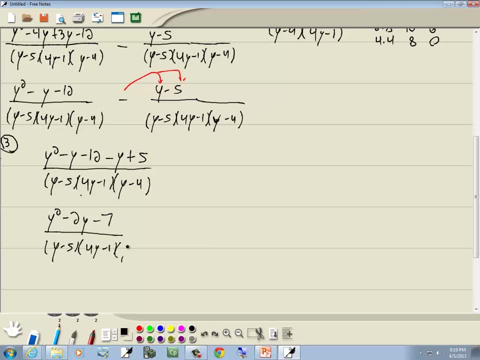 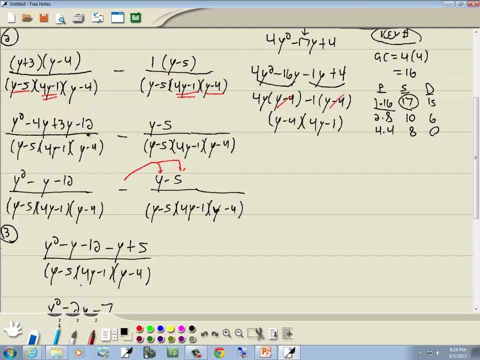 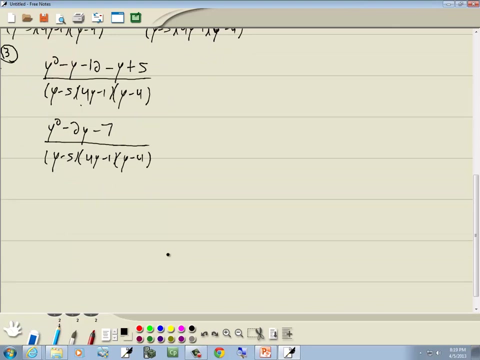 N. Negative 12 plus 5 is 0.. Ok, Add in the negative 보� firmware. Wait, Look at me. N. This is not a good one. I need to fix this. Let me double check. that Seems a weird answer to come up with. 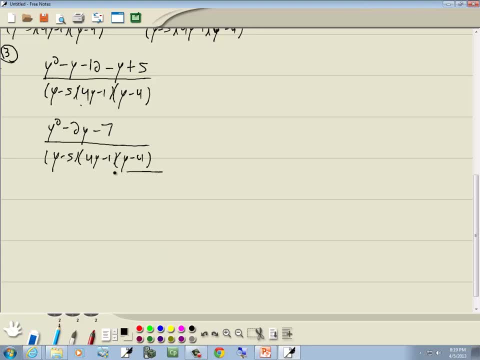 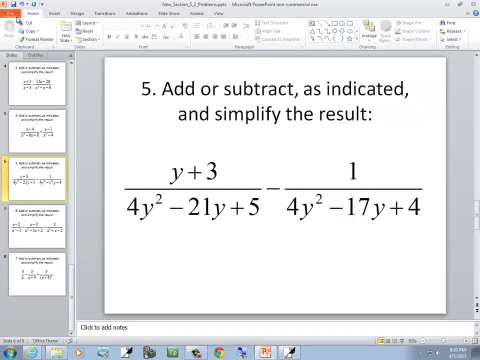 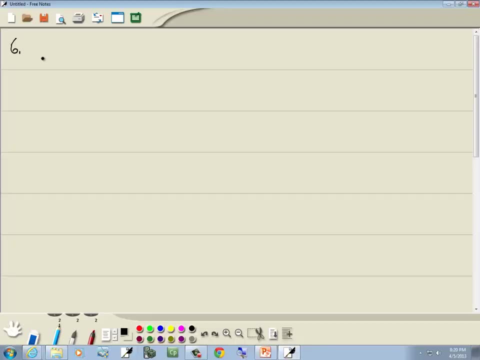 when I'm fading I'm kind of tired Way past my bedtime, 6.30.. Okay, let's look at our next problem. So we've got x minus 2 over x squared minus 1.. Minus x plus 3. 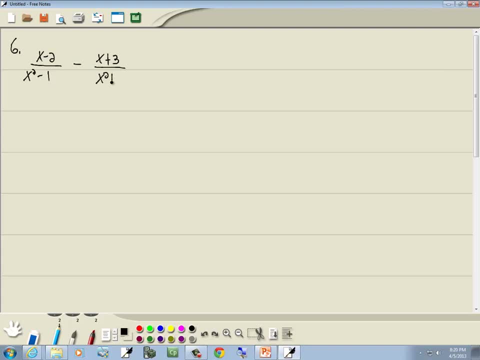 over x squared plus 3x plus 2 plus 3 over x squared plus x minus 2.. Well, our first step, Factor all of our denominators, This is dots Difference 2 squares Two terms of minus 3.. 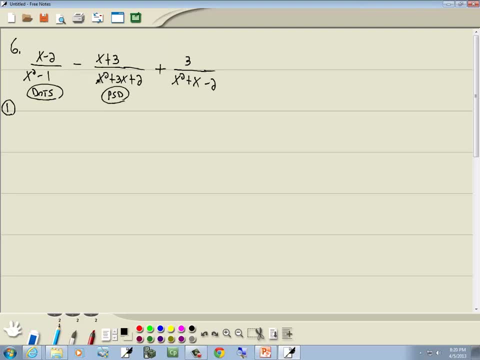 This one's PSD, Because we've got an x squared x, no, x, no number in front of the x squared. And this one's also PSD Because we've got x squared x, no, x, no number in front of the x squared. 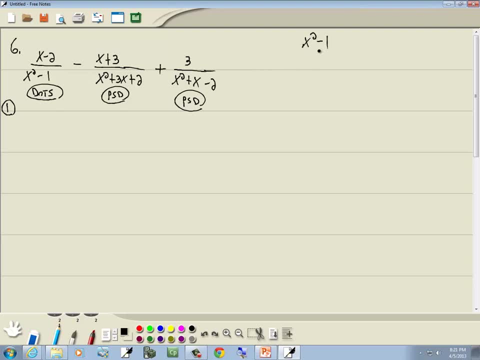 Well, let's look at the first one: The x squared minus 1.. Two terms of minus 3. You try to write it as something squared minus something else squared. You ask yourself what times self gives you the x squared? Well, x times x gives you x squared. 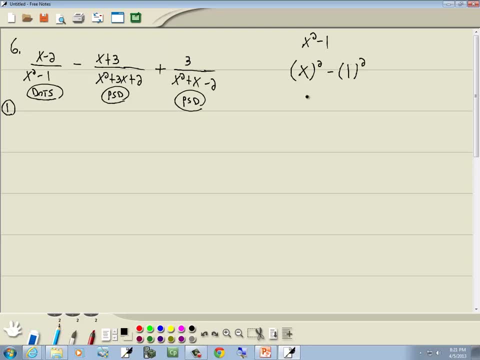 And what times self gives you the 1?? Well, 1 times 1.. 1 gives you that. So we take what's inside our first set of parentheses, We add what's in our last, And then you take what's inside your first and you subtract what's in your last. 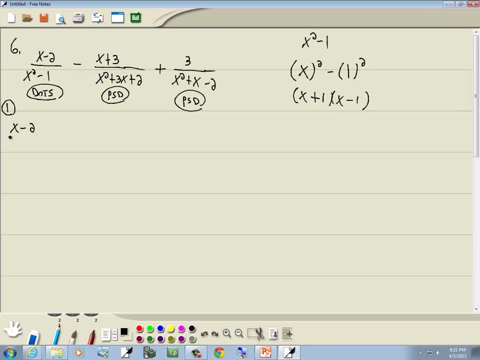 So this first part factors as x minus 2 over x plus 1, x minus 1.. Now the second one. here We've got x squared plus 3x plus 2.. PSD: we take the number at the end, which is 2.. 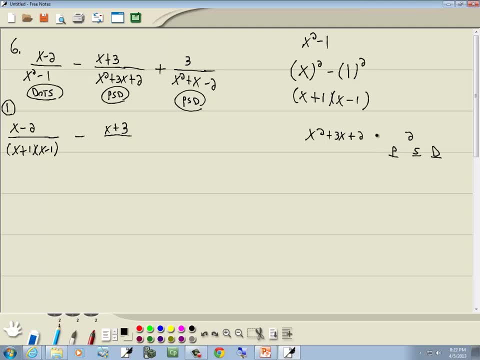 And we come up with our three columns. We write down all products: give us 2.. Well, 1 times 2.. We add them: 1 plus 2 is 3.. We subtract them: 2 minus 1 is 1.. 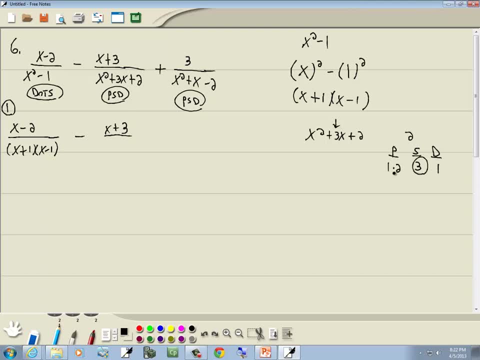 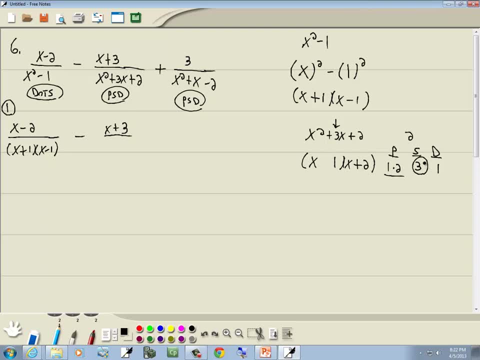 which is positive, The number. I circled in the S column S, for same sign. So if this is positive, then this is positive. So that's the way that factors. So this is x plus 1 times x plus 2.. 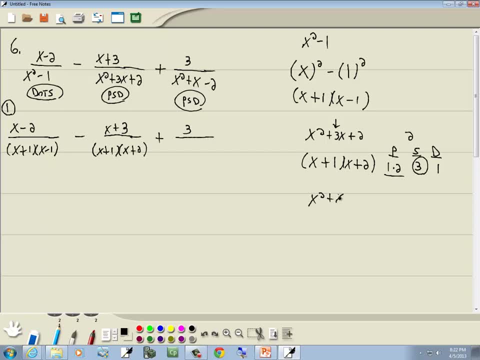 Now our next one. We have x squared plus x, minus 2.. And, as weird as it seems, we're using 2 again. So we're using the same table. The number we're looking for is the 1, which is over here. 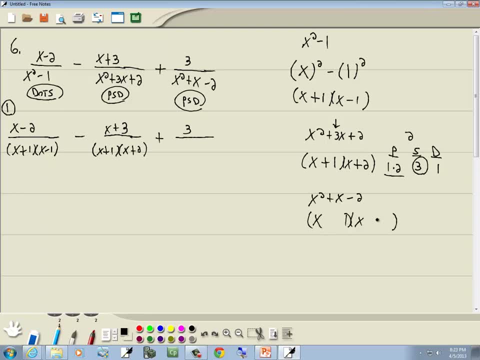 So we're going to have x, x, We use 1 and 2, again Our larger number, which is the 2,, which will always be the same sign as the middle term, which is positive. Now, the number we're looking for here is 1,, which is in the difference column. 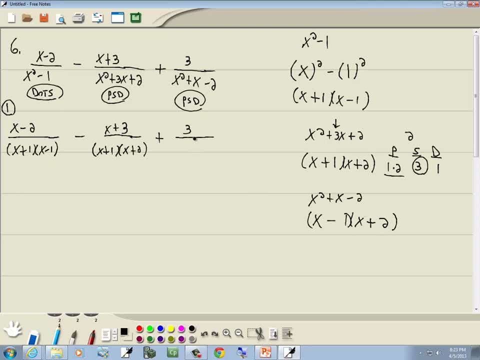 Which if this is positive, then the other one has to be negative, So that one factors this way. That seems weird just to have a 3 up there. Is that what I have? Yeah, just a 3.. Okay, step 2.. 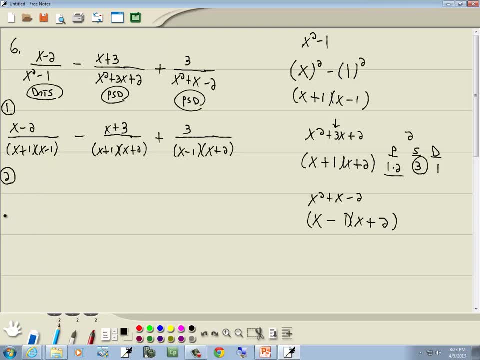 Figure out your least common denominator and rewrite each fraction with that new denominator. We'll start with our first. well, actually, let me put these down. We'll start with our first factor, the x plus 1.. We'll start with our first factor, the x plus 1.. 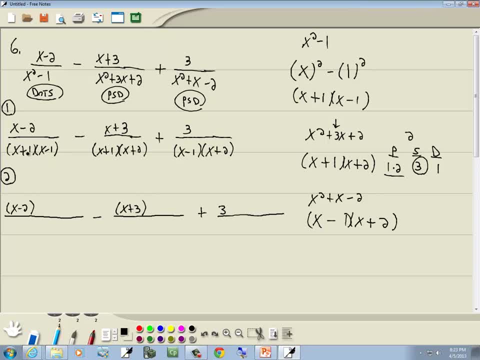 We'll start with our first factor, the x plus 1.. We're looking for the greatest number of x plus 1s in a single denominator. There's 1 here, 1 here, none here. So the greatest number of x plus 1s in a single denominator is 1.. 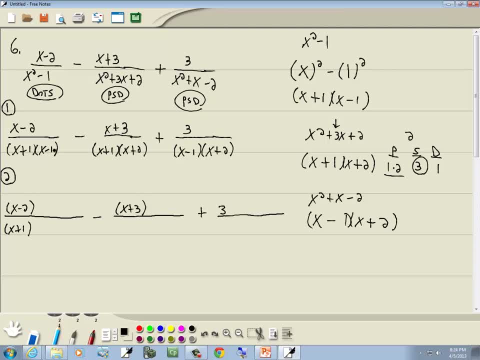 Then we'll go to our next factor, the x minus 1.. And we're looking for the greatest number of x minus 1s in a single denominator. There's 1 here, none here, 1 here. So the greatest number of x minus 1s in a single denominator is 1.. 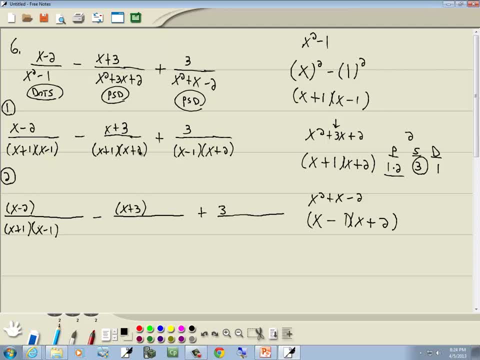 Then I'll go to my next factor, the x plus 2.. I'm looking for the greatest number of x plus 2s. So the greatest number of x plus 1s is 1.. Then I'll go to my next factor. the x plus 1s in a single denominator is 1.. Then I'll go to my next factor. the x plus 1s in a single denominator is 1.. Then I'll go to my next factor: the x plus 1s in a single denominator is 1.. There's none here, one here, one here. 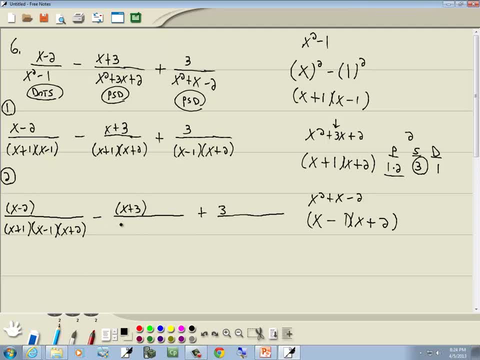 So it'd be 1.. So that's our LCD, And we're going to rewrite each fraction with that new denominator. Let me grab a drink here, Okay, Let's see what's changed. Let's see what's changed. Look, in our first fraction we had an x plus 1, the x plus 1 is still there. 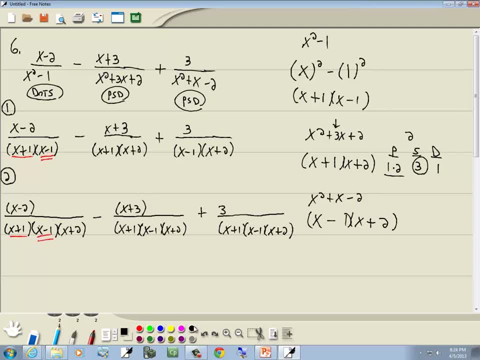 We had an x minus 1, the x minus 1 is still there. The new item down in the denominator is the x plus 2, so we have to put it up on top. On our second fraction, we had an x plus 1, the x plus 1 is still there. 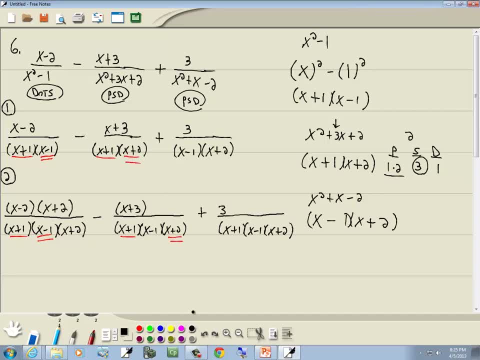 We had an x plus 2, the x plus 2 is still there. The new item downstairs is the x minus 1, so we have to put it up on top. And then our last fraction here: we had an x minus 1, the x minus 1 is still there. 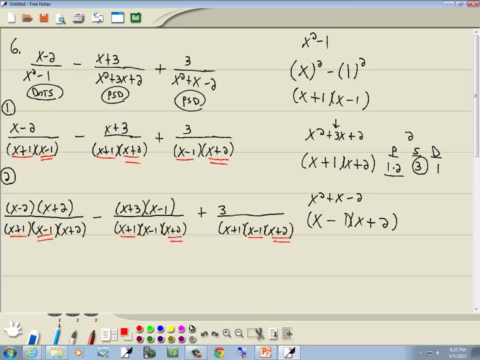 We had an x plus 2, the x plus 2 is still there. The new item down in the denominator is the x plus 1, so we have to put it up on top also. Whatever you multiply by the bottom, you have to multiply by the top. 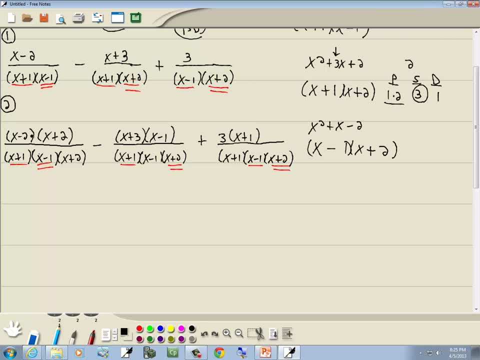 Okay, now I'll multiply these together. These are conjugates, so I can make this a little bit simpler, but let me pretend I don't see that x times x is x. x squared, x times 2 is 2x. 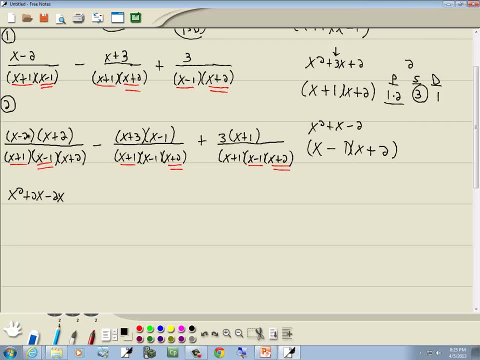 Negative 2 times x is negative. 2x. Negative 2 times 2 gives us negative 4.. Over our denominator: Minus x times x is x squared. x times negative: 1 is negative. 1x. 3 times x is 3x. 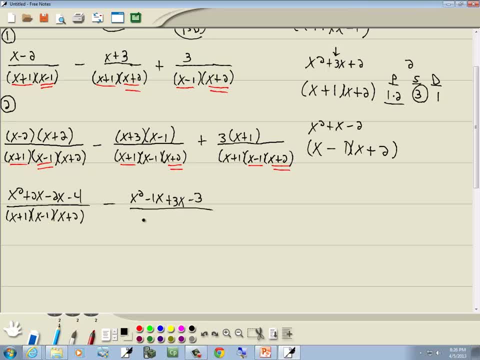 3 times negative. 1 is negative. 3. Over our denominator: Over our denominator, And this is a distributive property here, 3 times x is 3x And 3 times 1 is 3. Over our denominator. 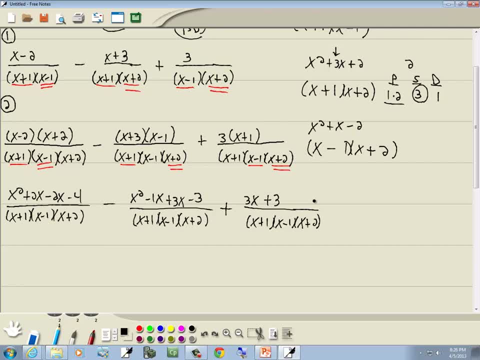 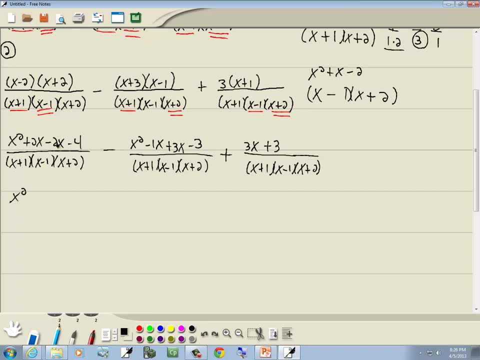 Okay, Well, let's combine together like terms. So we're gonna have x squared 2x minus. 2x drops away. so we got x squared minus 4 over our denominator Minus. Then x squared Negative 1x plus 3x gives us a positive 2x minus 3 over our denominator. 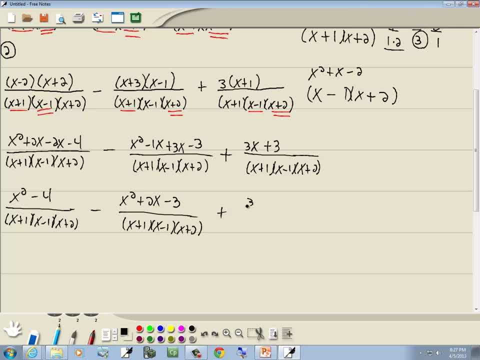 Plus 3x plus 3x. Minus 3x Over our denominator x. plus three over our denominator. Okay, now we're ready for the next step. We want to merge these into a single fraction by adding or subtracting the top parts. Now remember. 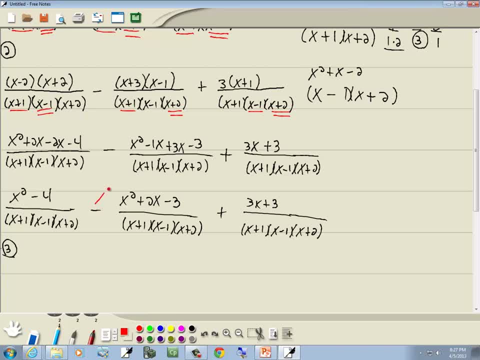 if you have a negative out in front of your fraction, that negative is going to flip a sign of all the terms up on top. So this negative here is going to flip a sign of the x squared of two x and negative three. So we're going to have x squared minus four minus x squared. 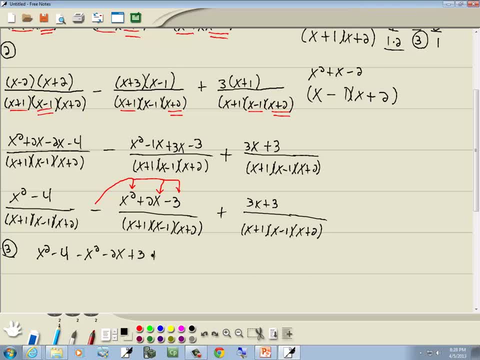 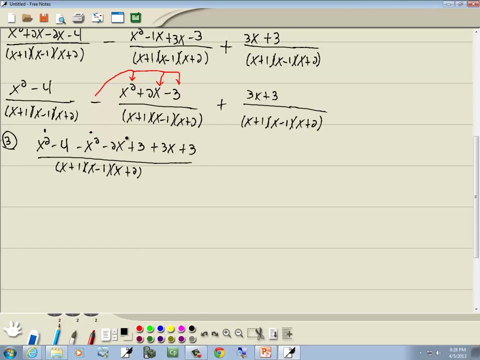 minus two, x plus three plus three, x plus three all over our denominator. Okay, combine together like terms: x squared minus x squared cancels. Here we got negative. two x plus three, x, that gives us x, Here we have a negative. four plus three is negative. 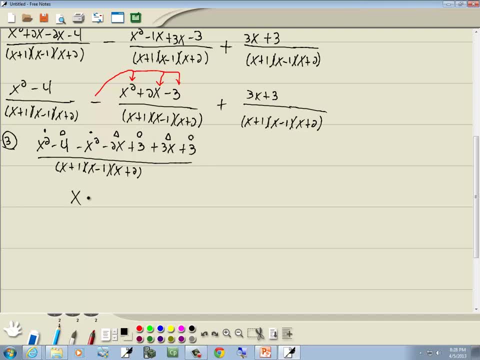 one plus three gives us two, So we got x plus two. Okay, step four: factor your top, factor your bottom. Well, the top and bottom are both factored as much as they can be. So step five: cancel, if possible. See how we have an x plus. 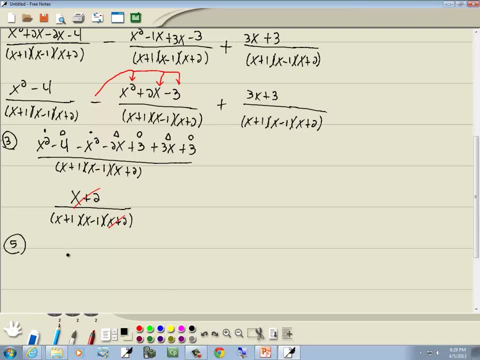 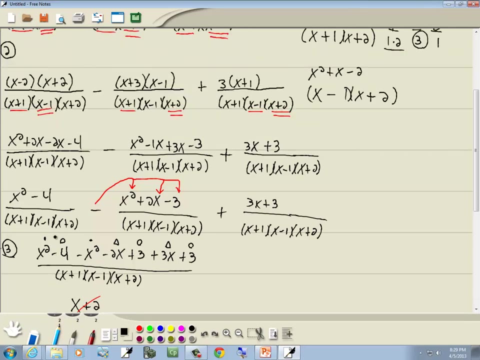 two here and we have an x plus two here. Those are going to cancel and we're left with one over x plus one times x minus one. Now, one thing I want to mention up above here is when conjugates means the first and the second are the same, the sign in the middle is different. 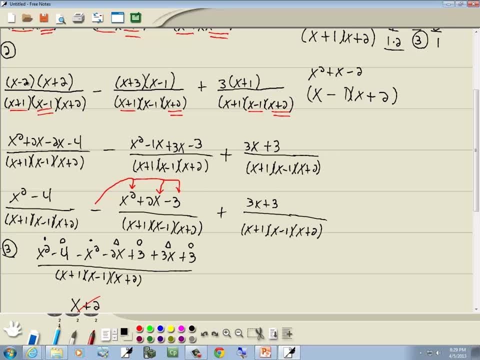 See how the x minus two times x plus two. they both start with x and they both have a two at the end, But this one has a minus between them and this one has a plus between them. When you got conjugates, all you have to do is multiply your first parts together and 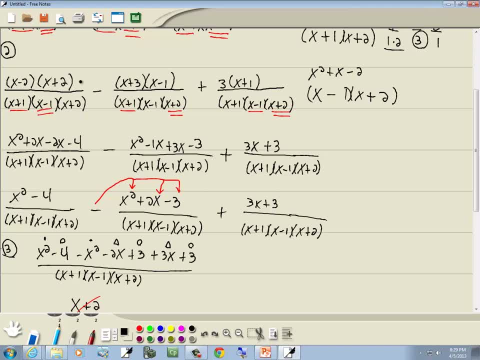 your last parts. So x times x is x squared, and negative two times two gives you negative four. So it saves a little bit of work. if you recognize that Now, you'll notice. if you don't recognize it, you still get the correct answer. 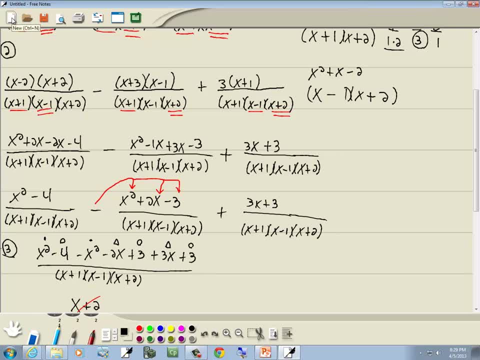 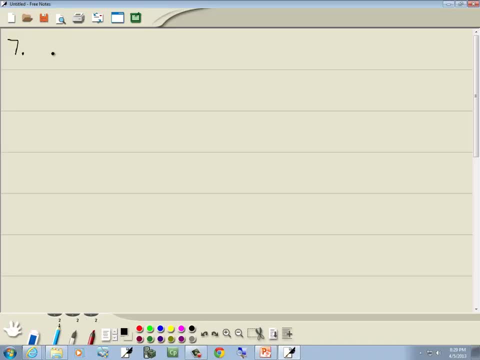 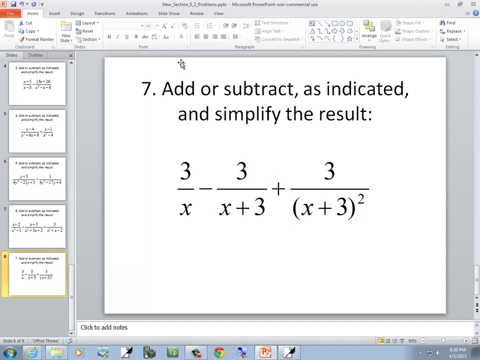 And let's look at this last problem. Okay, so we got three over x minus three over x plus three plus three over x plus three squared. Well, step five: cancel, if possible. See how we have an x plus two times x minus one times. 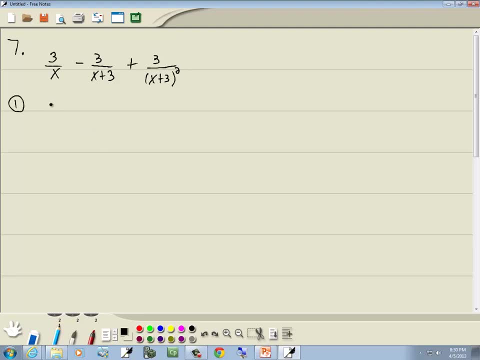 two. Step one: factor all your denominators, This would become three over x minus three over x plus three plus three over x plus three times x plus three. That's what that x plus three squared means. Step two: figure out your LCD and rewrite each fraction with that. 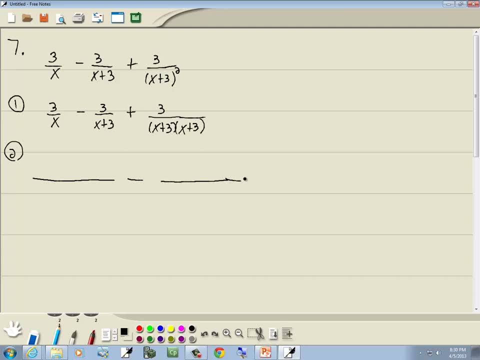 new denominator. Well, realize that a single x here is different than x plus three. So we'll start with the x. I'm looking for the greatest number of single xs in a single denominator. There's one here, none here, none here. So greatest number of single xs in a single denominator. 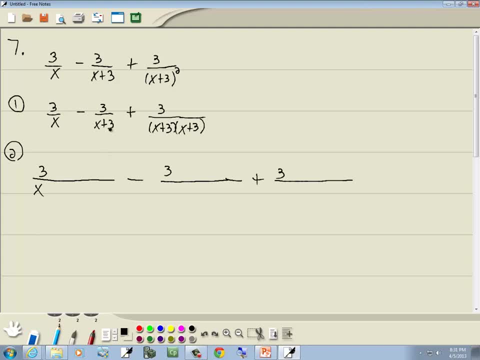 is one. And then I go to my next factor, the x plus three. I'm looking for the greatest number of x plus three a single denominator. there's none here, there's one here, there's two here. so the greatest number of X plus 3 is in a single denominator, is 2. so that's our. 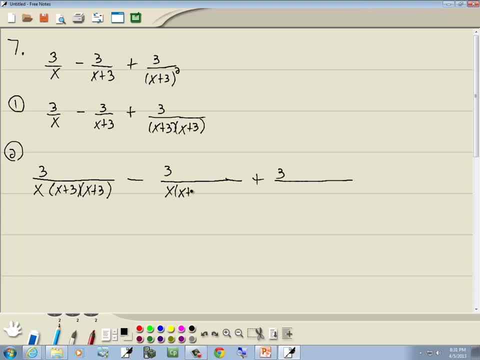 LCD and we're going to rewrite each fraction with that new denominator. okay, now we're going to look at our old denominator and see what's changed. well, we had an X here. the X there is still there. the new item we put down denominator is the X plus 3, X plus 3. so whatever we put down there we have to put up on top. now our second fraction. 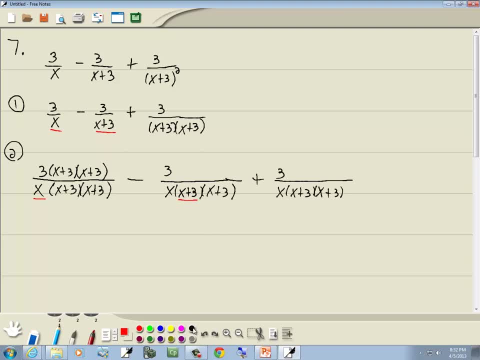 we had an X plus 3. that X plus 3 is still there. the new items downstairs is the X and the other X plus 3, our last fraction. we had an X plus 3. that's still there. we had another X plus 3. that's still there. the new item downstairs is the X. 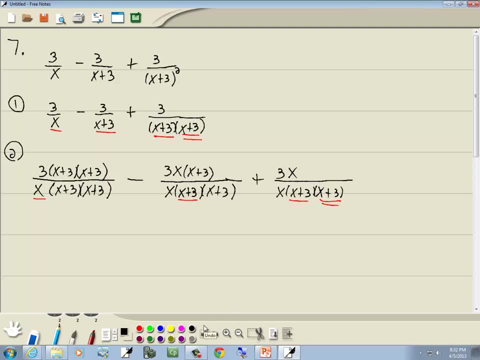 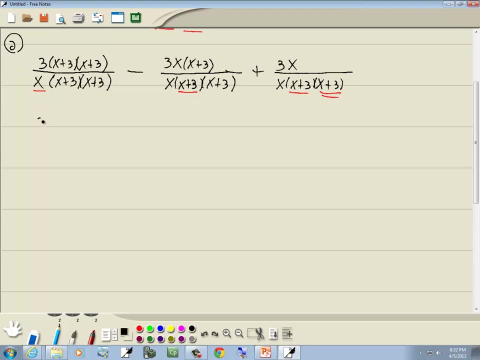 so put that on top. well, let's go ahead and multiply together the um what's up in numerator top. so here we got X plus 3 times X plus 3. 3, x times x is x. squared x times 3 is 3x. 3 times x is 3x. 3 times 3 is 9, over our denominator minus. this is a distributive property. we'll take: 3x times x is 3x. squared 3x times 3 is 9x over our denominator. 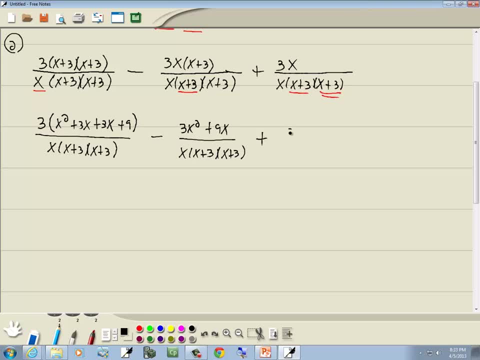 Plus 3x over our denominator. Well, combine the alike terms here. so we got x squared. 3x plus 3x is 6x plus 9, and then everything else remains the same. So I'll go ahead and write it all down. 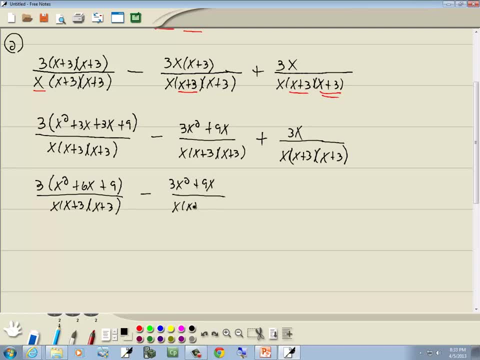 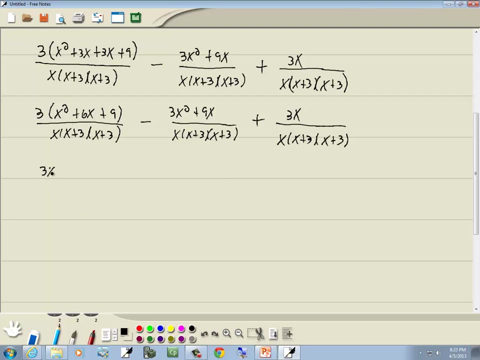 So these problems make your hands hurt from writing, Okay, well, back to our first fraction. We'll multiply the 3 through 3 times x. squared is 3x. squared 3 times 6x is 18x. 3 times 9 is 27.. 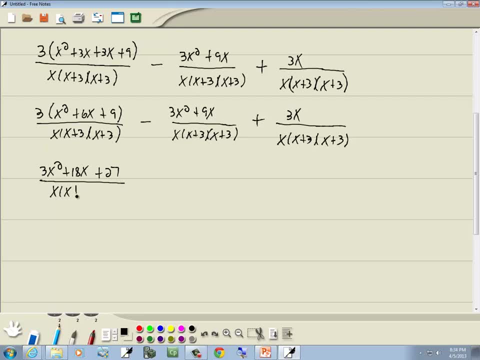 Over our denominator And everything else remains the same. so I'll go ahead and carry it all through. And that was step one. Okay, step two. We want to add or subtract. We want to subtract our top parts and merge them into a single fraction. 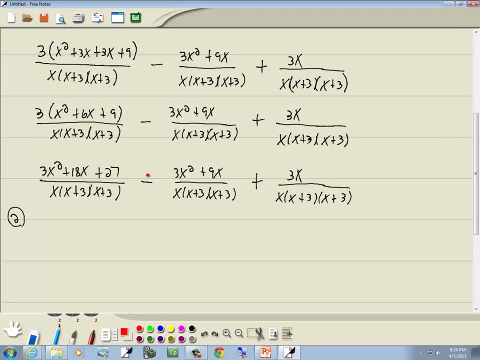 Remember, if you have a negative out in front of your fraction, it's going to flip the sign of all the terms up on top. So it'll flip the sign of the 3x squared and the 9x. So this is going to become 3x squared plus 18x plus 27,. minus 3x squared minus 9x plus 3x. 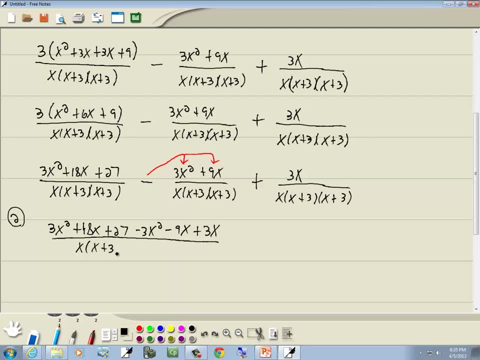 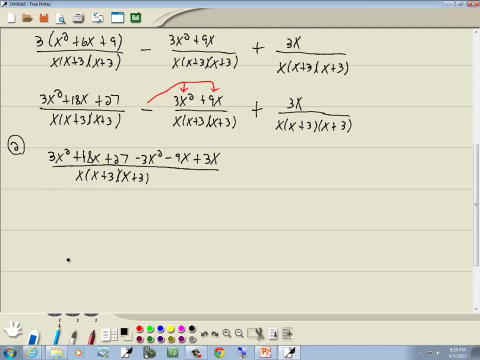 all over And that's our denominator. Well, combine together like terms. We have 3x squared minus 3x squared. that cancels. We have 18x minus 9x plus 3x. Well, 18x minus 9x is 9x plus 3x is 12x. 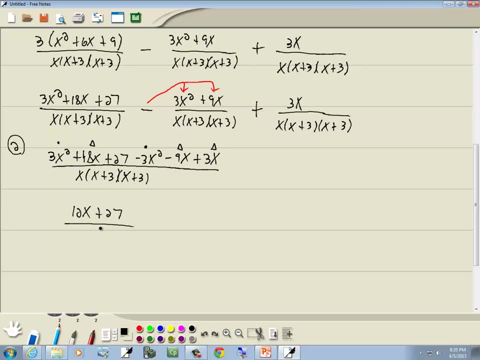 And then the plus 27.. You're going to divide it by six Every 20 times, Another 20 times, Huhh, Every 10 times. Let's have some more representation on there. I think I'm off with my numbering here, aren't I? 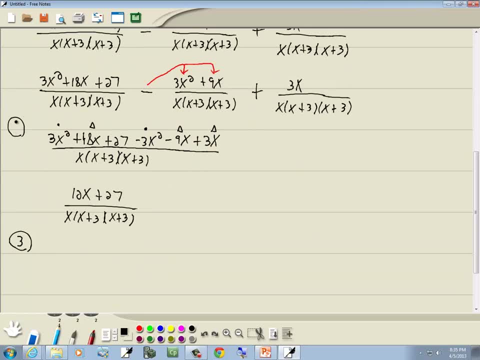 Okay, that should be step three. Time for bed. This is step four. Okay, Step four: Factor, your top Factor, your bottom Stop, GCF. They both least have a 3 in common, so I'll factor out a 3, and that gives us 4x. 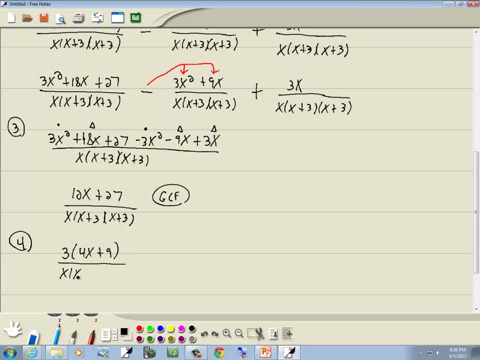 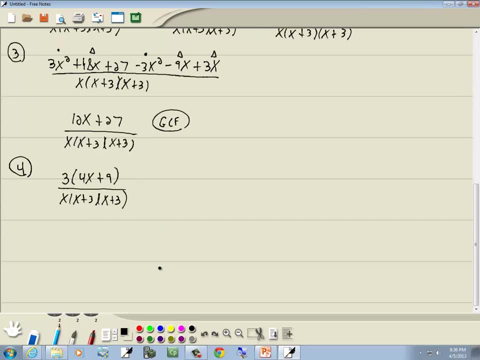 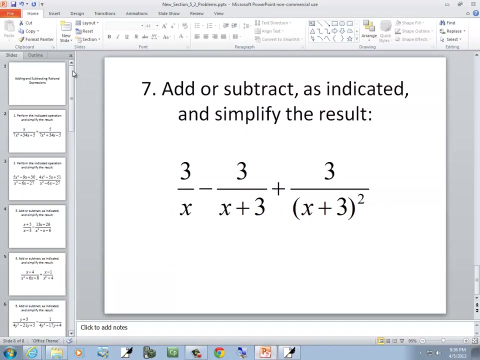 plus 9.. Now step 5 says cancel if possible. Well, there's nothing to cancel here. Now the way they will write their answer is they'll write this as x times x plus 3 squared. But that would be your answer. I believe that was the last problem, so I'll stop the little. 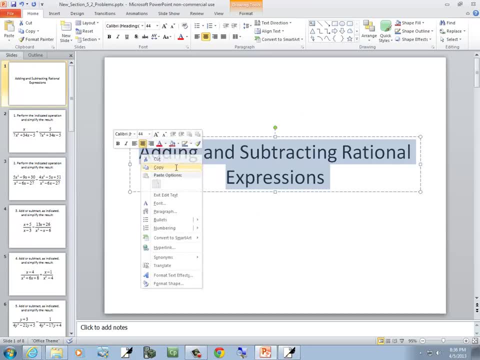 video Adding and subtracting rational expressions. 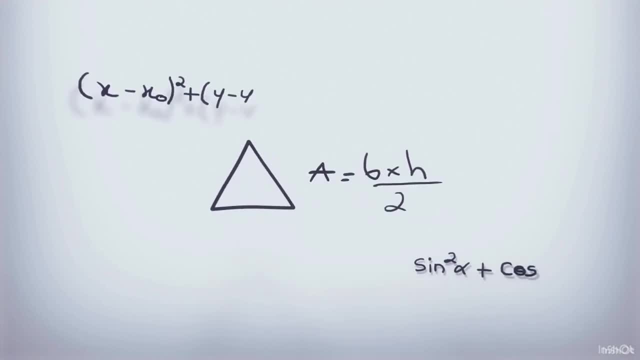 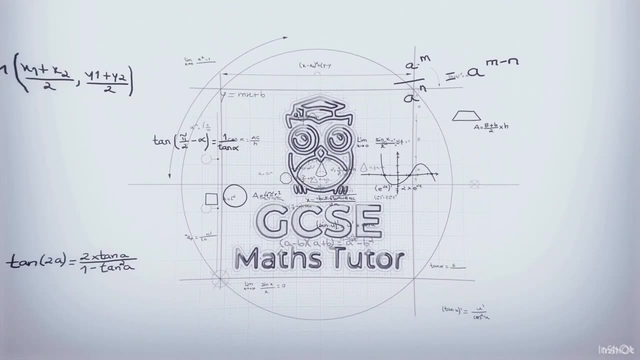 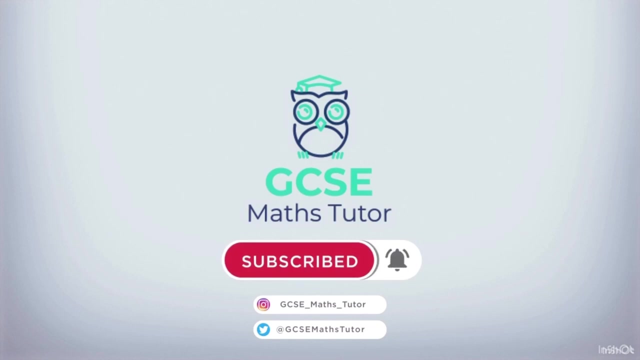 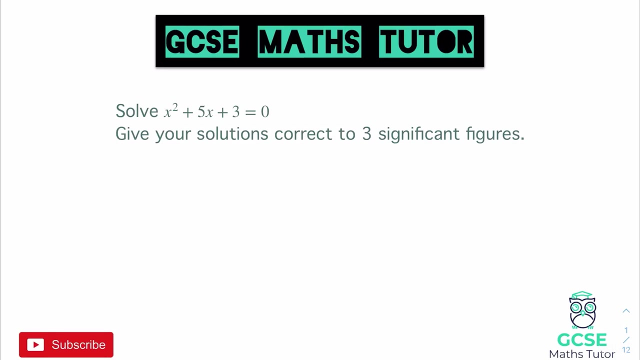 Okay, so in this video we're going to have a look at the quadratic formula and how to use it. Now we're going to have a look at mostly calculator questions with a few different types of examples, and in the final few we're going to have a look at some non-calculator examples and